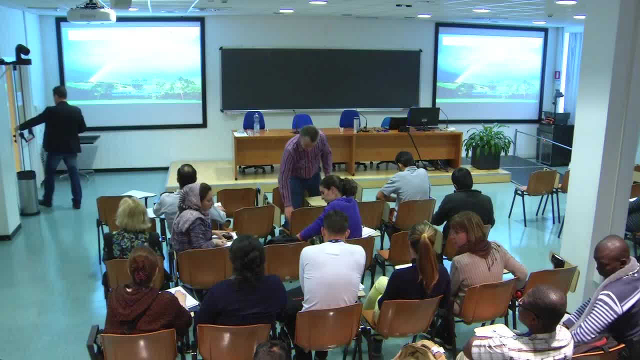 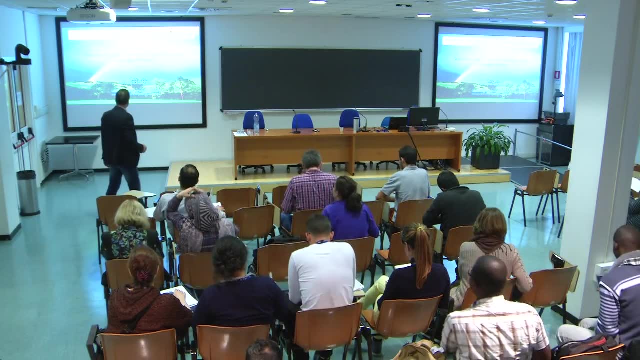 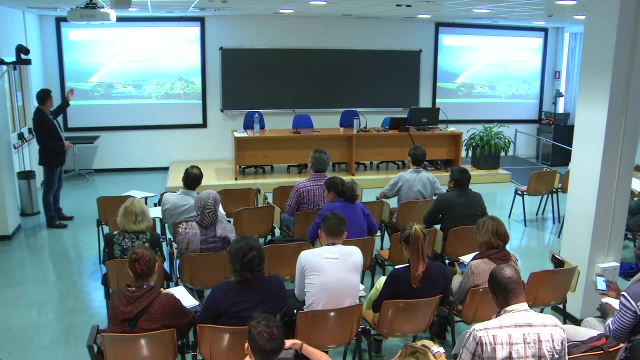 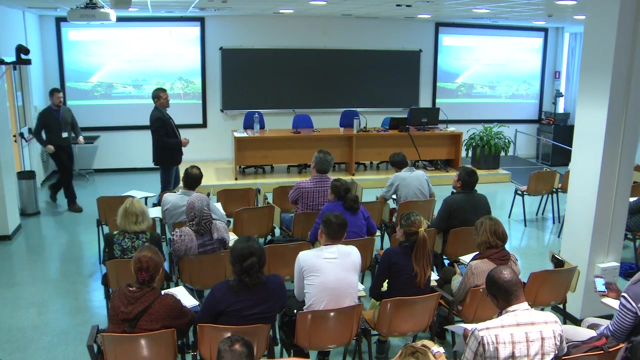 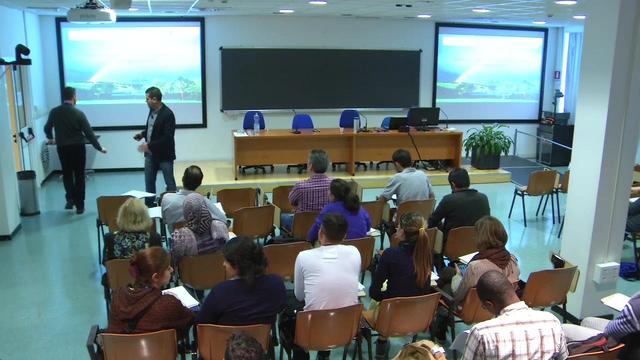 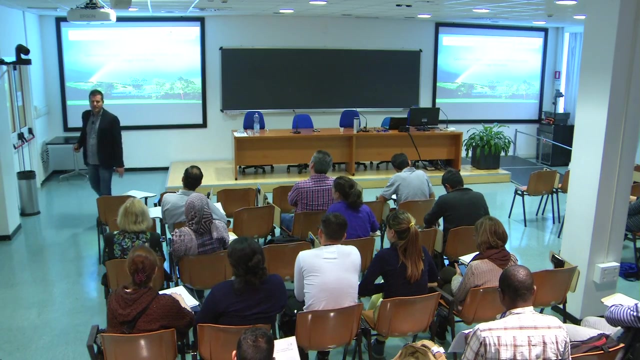 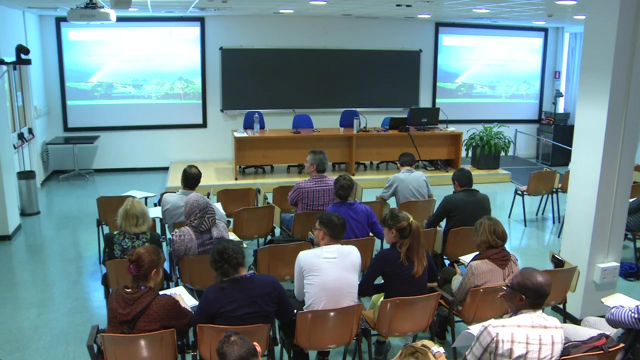 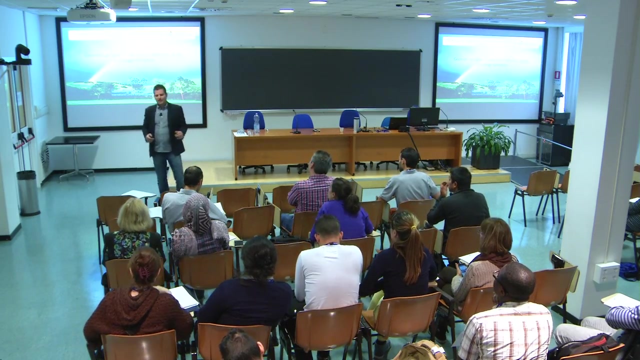 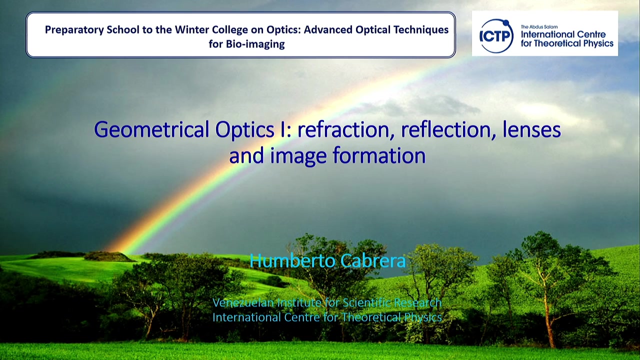 Thank you. Okay, let's restart with this conference. that is very, very basic. Miguel will continue with this context and you will see that we will repeat again and again, because it's very important for you to know about these lectures, because this is a very important conference. 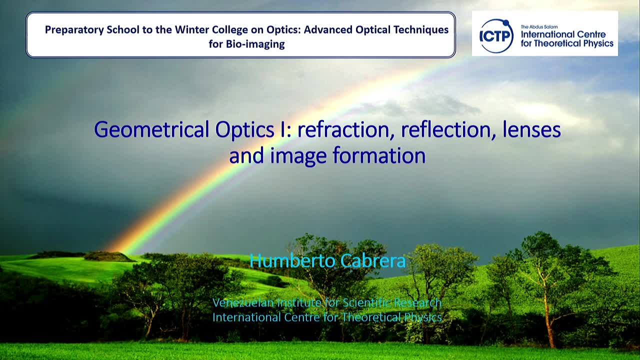 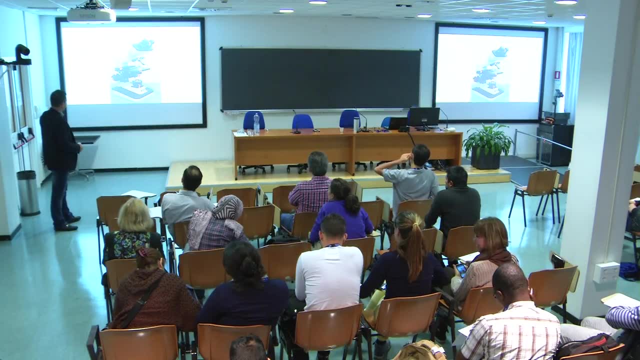 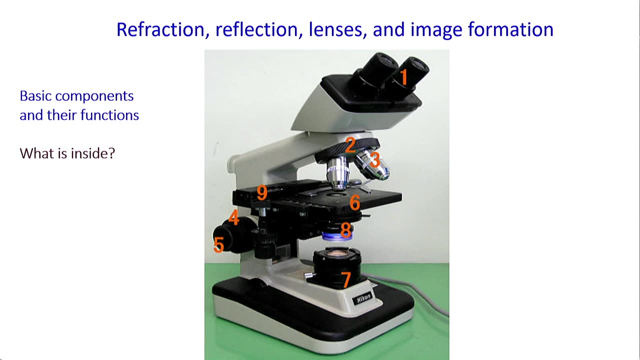 This is what you will see in the lab, This is the basis of all the lectures, and so on. Then, as I say to you, a microscope is built with different lengths, but not single lengths. We will derive the theory of microscope using thin lengths, using single lengths. 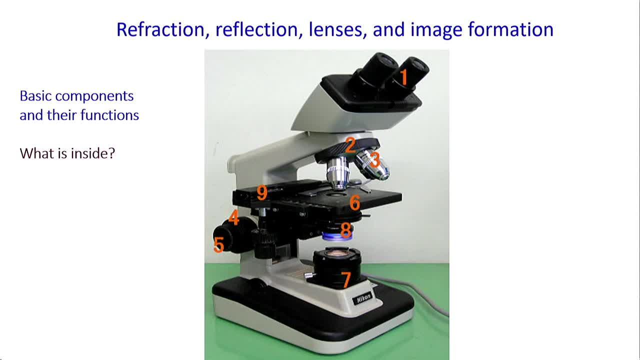 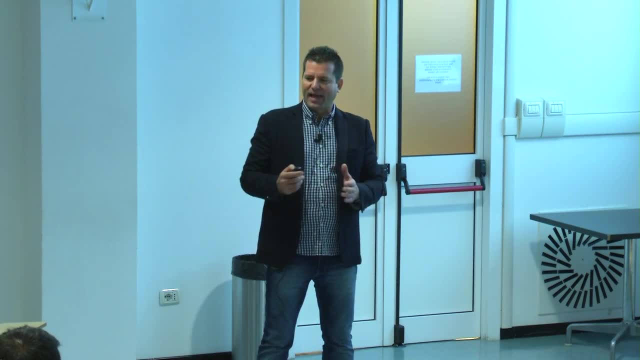 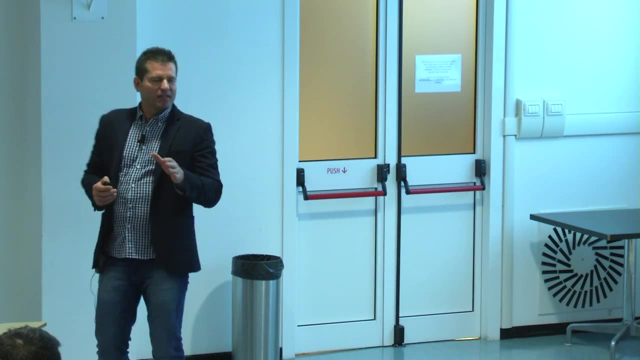 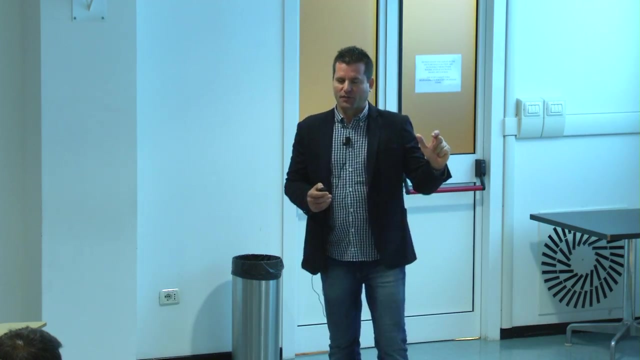 but in real, In the world. the microscope objective is a complex set of lengths, but the theory of a single length applies for this. You only need to know some basic concepts- lengths make an equation, image formation with different lengths- and then you can apply this to the microscope objective. 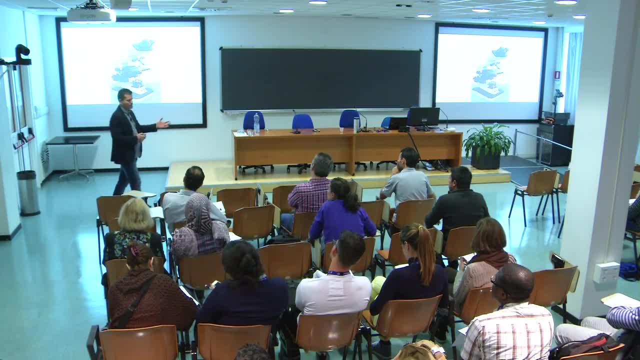 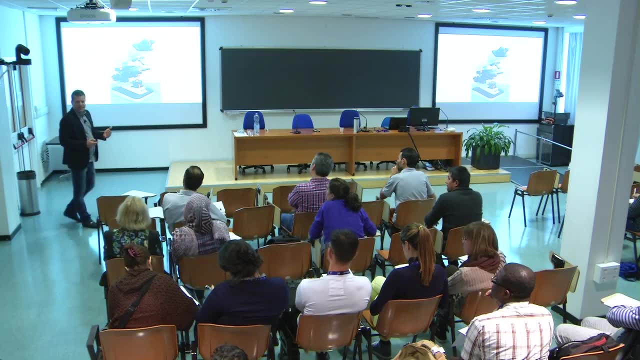 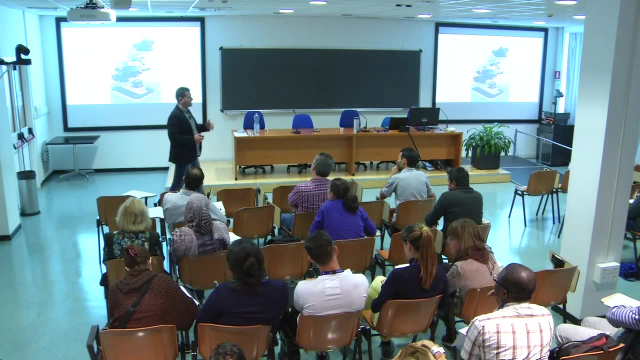 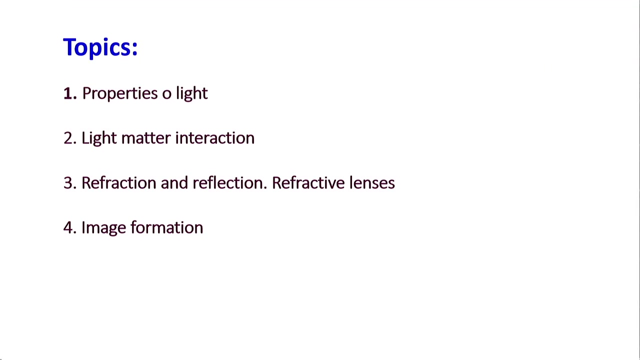 And also we will have a lecture about microscope objective And also we will have a lecture about microscope objective Tomorrow, about a solution. but to understand what is inside a microscope, we need to know this complete theory. We need to know about the properties of light and how the light interacts with matter. 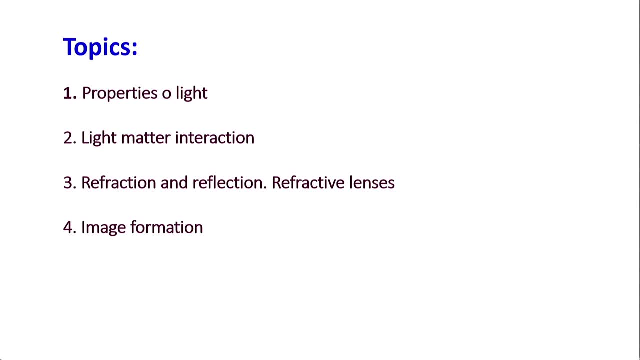 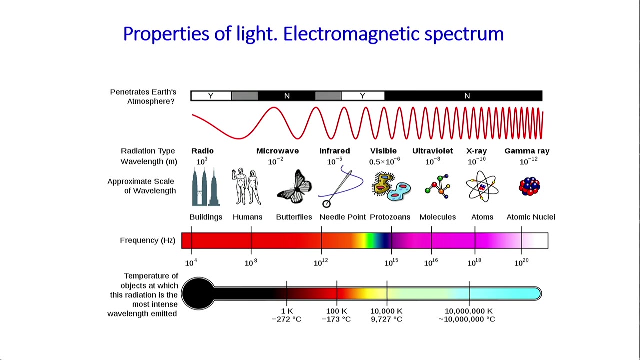 This will answer some of the questions asked you gave before, also about refraction and reflection, refractive lens and finally, about image formation. Let's start with a very, very simple figure about the electromagnetic spectrum. We know that the electromagnetic spectrum the human eye is only able to capture. very 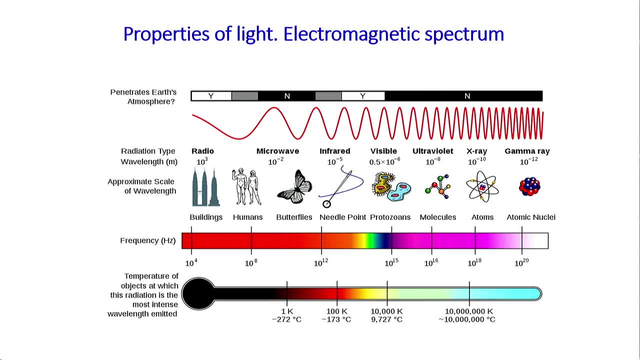 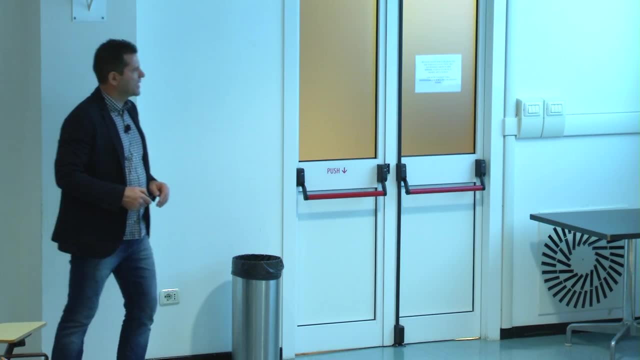 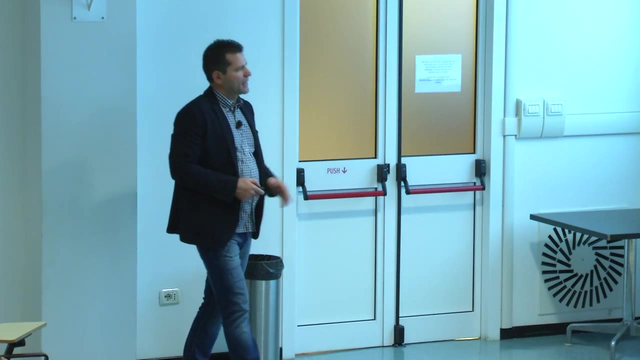 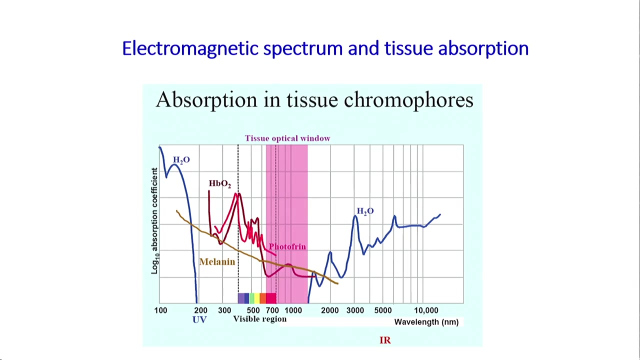 very small regions of this spectrum here in the visible 400 to 700 nanometers. Different animals have different vision, But also we are showing here different scales to compare with the light and also with microscopy. But also it's very important when we use microscopy, for example fluorescent microscopy or optical 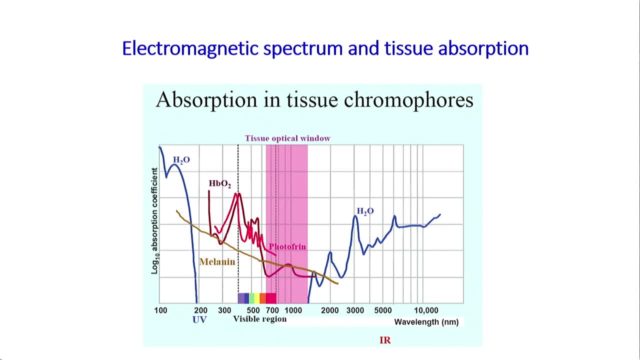 tweezers to know about the absorption of our skin. For many medical applications using lasers and light. this is very important because, for example, we have here in this figure we can see how different components of the skin absorb, for example, water in the UV region of the spectra. also, 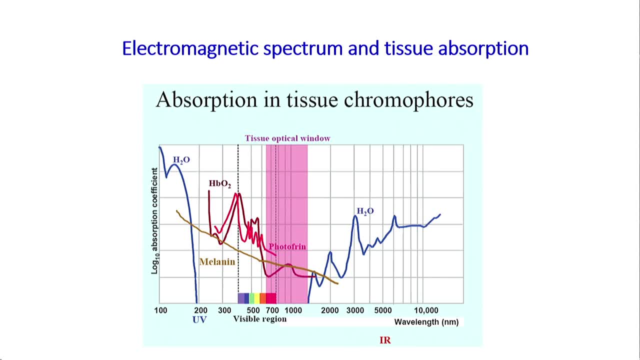 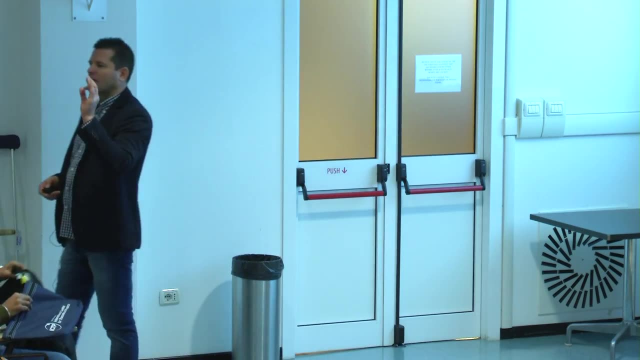 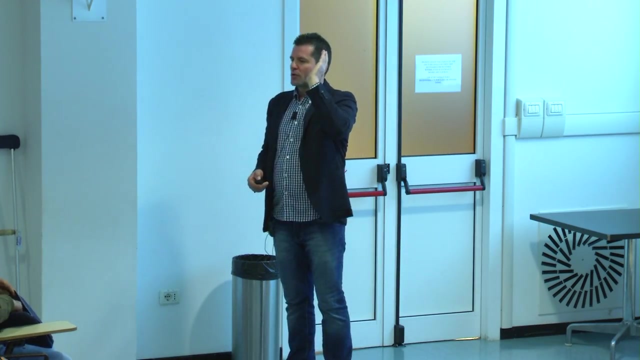 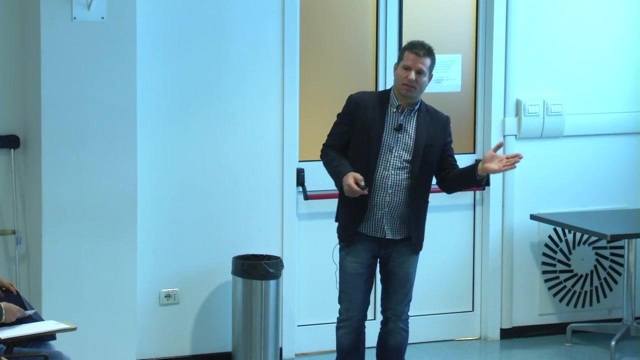 in the infrared Different components- hemoglobin, melanin, photofrein and so on- and this makes that in this region between 700 and 1 micron we have the optical window for humans, especially the skin. Due to that, normally we use for manipulating cells. for laser depilation we use 900 nanometers. 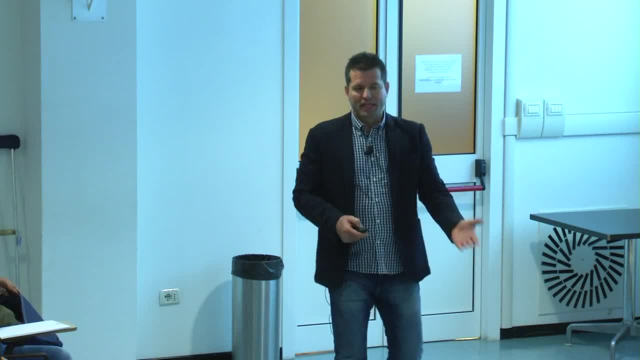 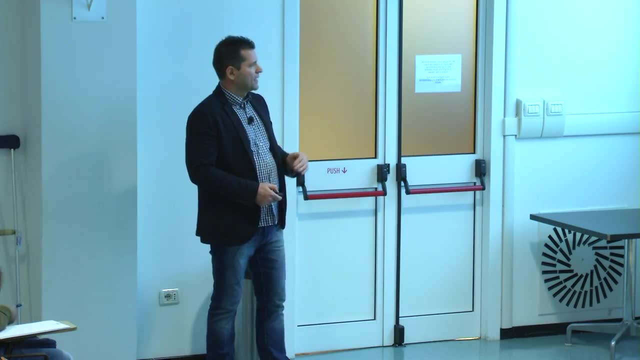 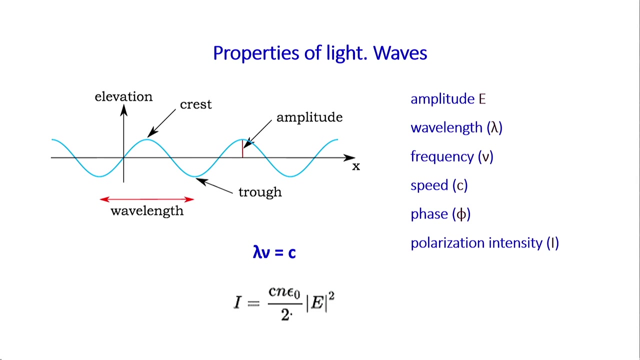 because there is less interaction with the skin and the damage will be decreased. Also the properties of light, Because we will derive also here in my course and also in Miguel's course about the ray theory but also about the wave theory, Because, as I said to you before, in microscopy, mainly in image formation for deriving very 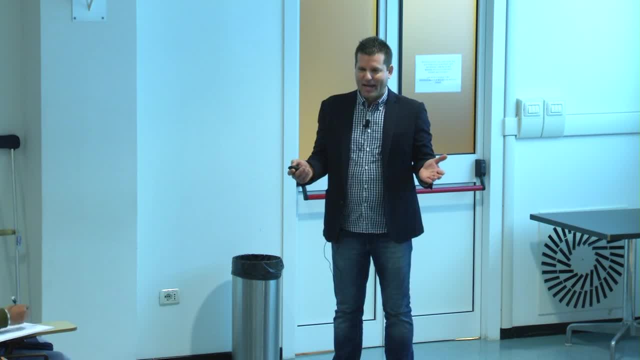 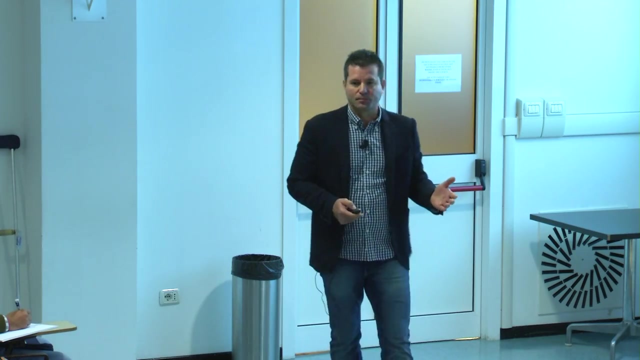 very simple equation, that we use ray optics, but for the deriving there, for example the point spread function, We need to know about wave optics, for image formation, for aberrations and so on. Due to that, it's very important to know the main or to remember you. 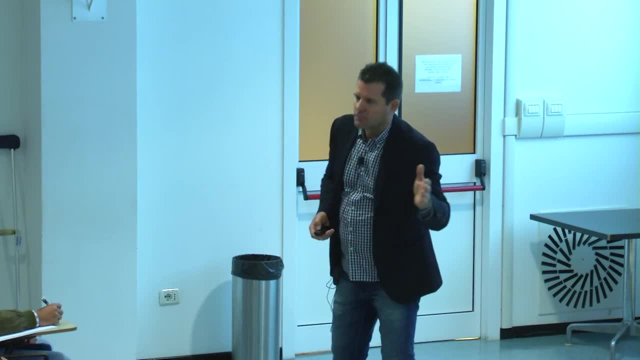 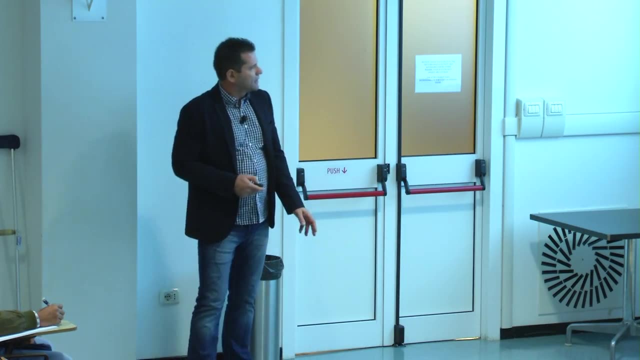 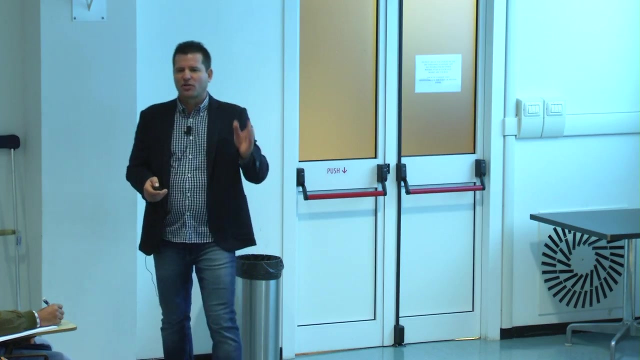 because I know this is very basic, maybe for many people here, but maybe for others no, and we have to remember this. The line is an oscillation, not physical oscillation. It's oscillation of the electric field and magnetic field in space. sinusoidal variation. 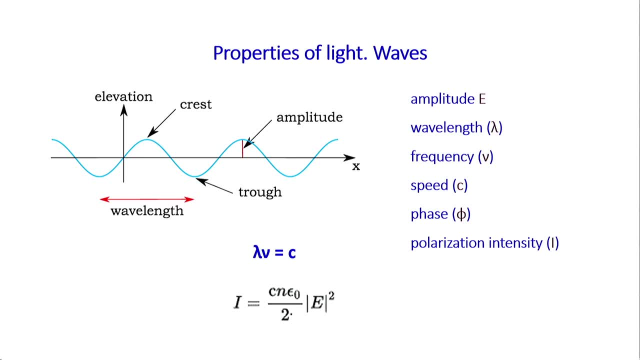 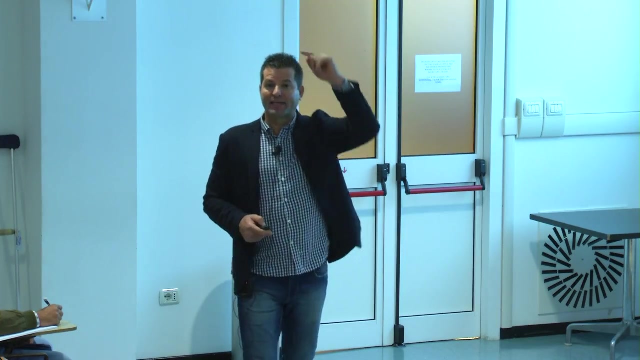 This wave has amplitude. this is the amplitude of the electric field Wavelength. the wavelength is the distance between to minimum or to maximum. We also have frequency. this is the inverse of the wavelength. Speed of light phase. Depending on this oscillation when it's starting in the space. 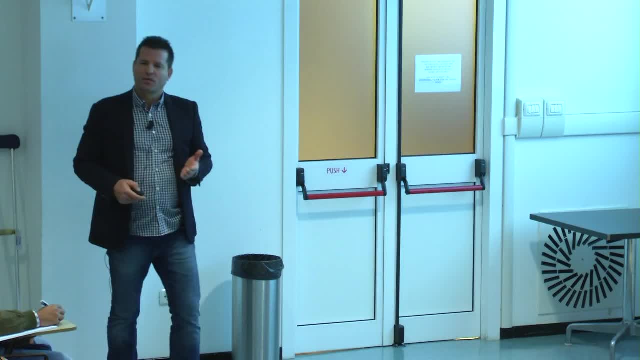 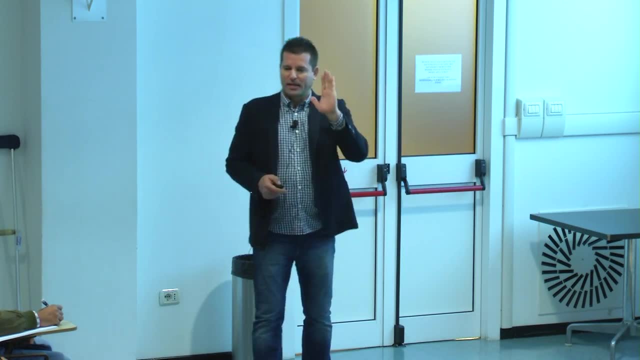 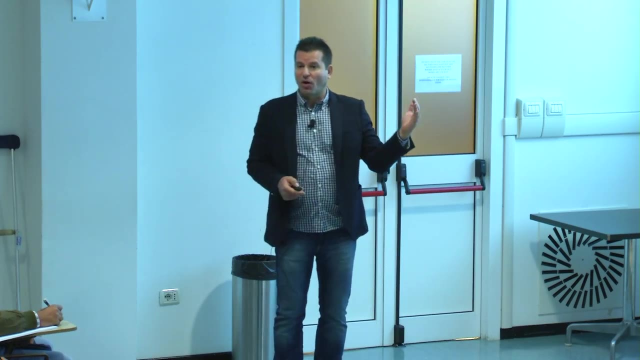 And also we have polarization intensity. For example, the laser, the helium laser, are mainly polarized in some direction, For example. it's very important for polarization microscopy to know about this concept, But there is a very, very basic equation that relay this parameterization. 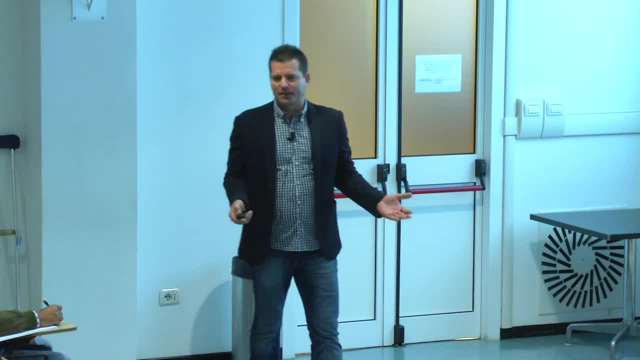 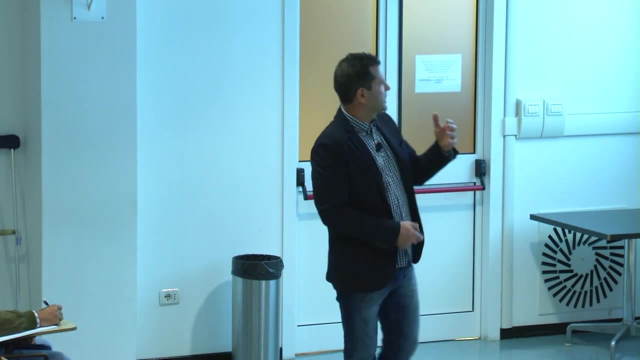 So it's the temperature, the wavelength, the frequency and the speed of light. This equation, And also the electric field, is related with the intensity. through this relation, Our eyes are not able to detect this very, very fast variation: 10 to 14 hertz. 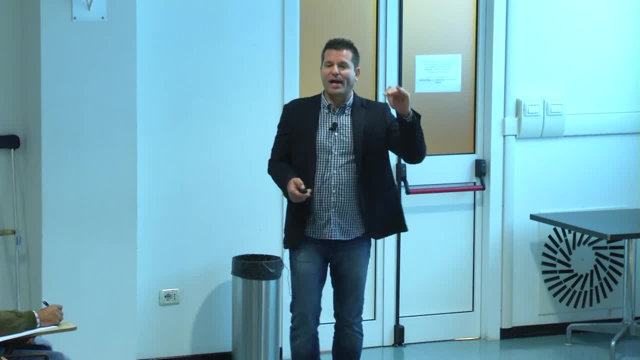 Only reacts, and detectors, of course, react to the square of this field And, due to that, we will use mainly the intensity And, due to that, we will mainly use the intensity And, due to that, we will mainly use the intensity. 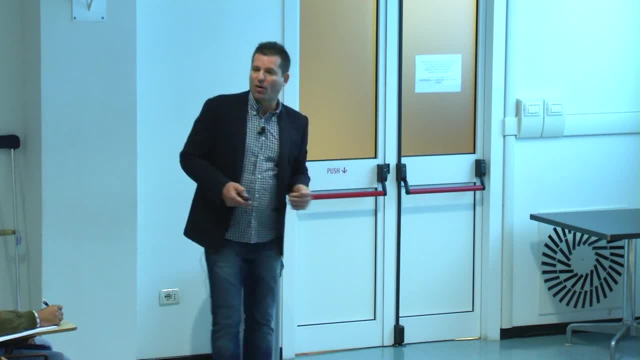 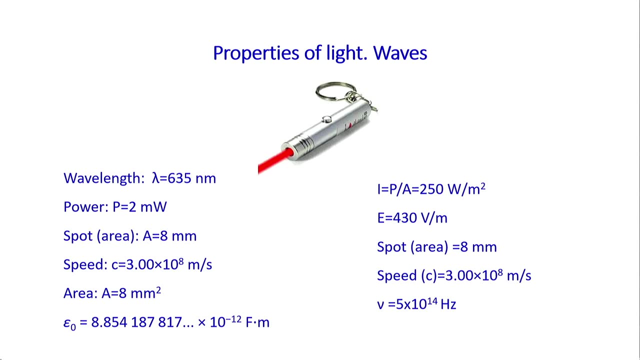 And due to that we will mainly use the intensity. This is the strength of the electric field, intensity of light as a square of the electric field. But let us show you an example that is also very common in many applications: in medical applications and also in biological applications. 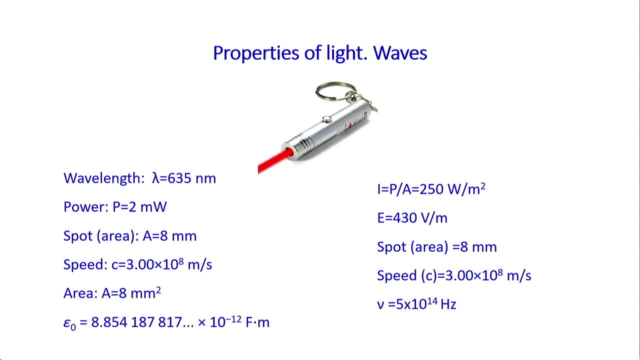 You must know about very important parameters and, of course, when you look at the paper, this is the main parameters reported there. Let's we look at very, very simple laser pointing, okay, With a wavelength 635 nanometers, with a power 2 milliwatt, a spot area, this spot area onto. 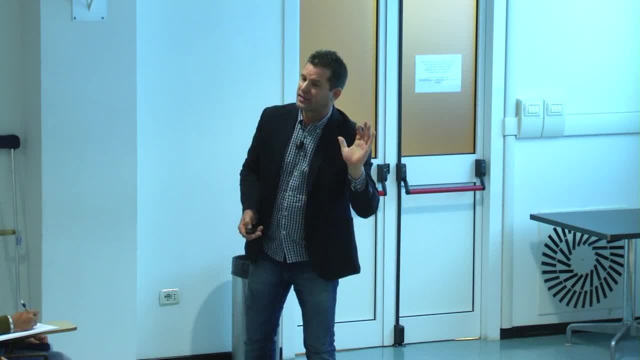 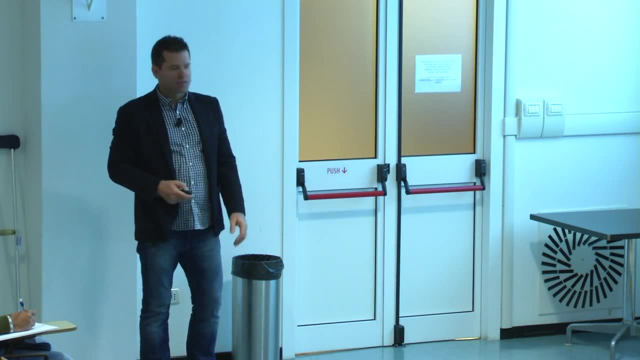 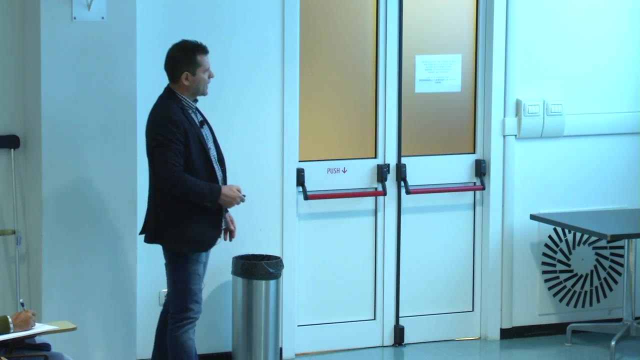 the sample. Of course you can't concentrate with the lens and you will take this spot area. You increase or reduce the power density, But let's we take this. This is a small 8 millimeter spot. Of course the speed of light is also necessary here with this area and the electric constant. 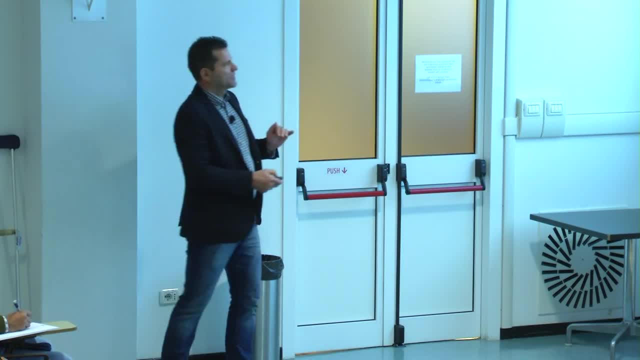 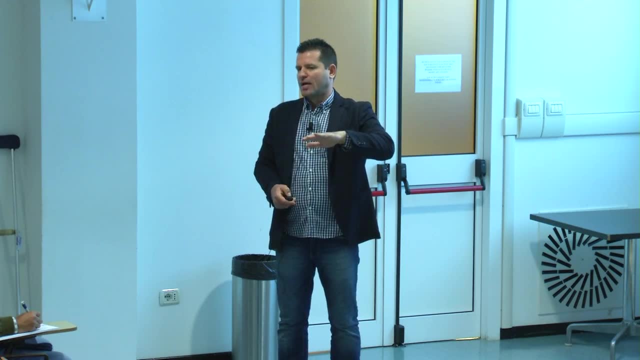 The electric constant And with this we can calculate, for example, the intensity or the irradiance. Some people say irradiance, Some people say intensity. I say irradiance because intensity is also used, taking into account for the angle and irradiance. 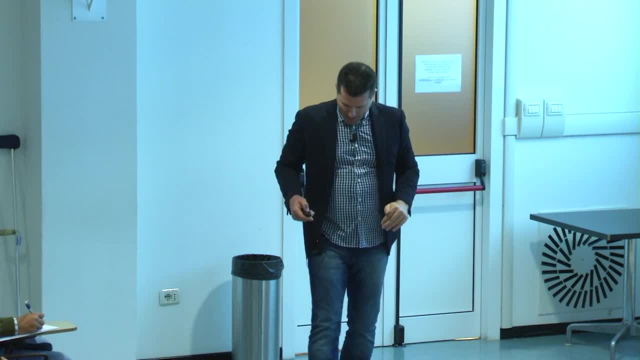 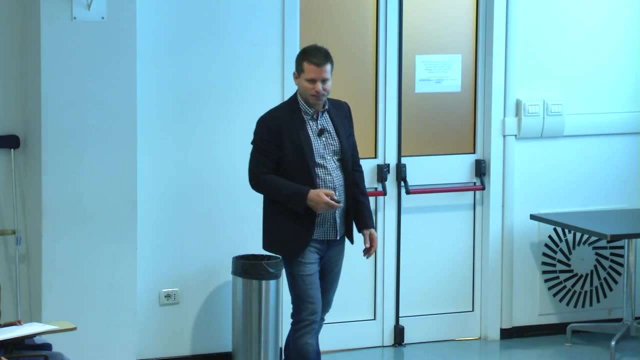 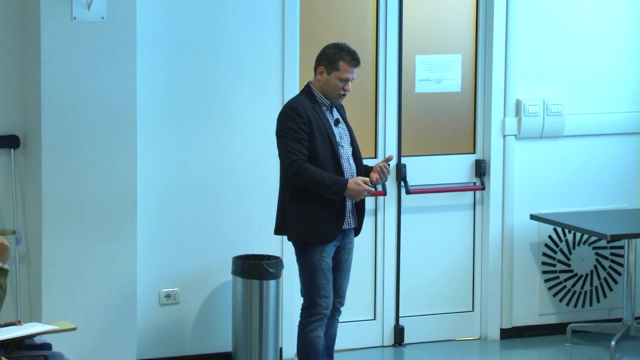 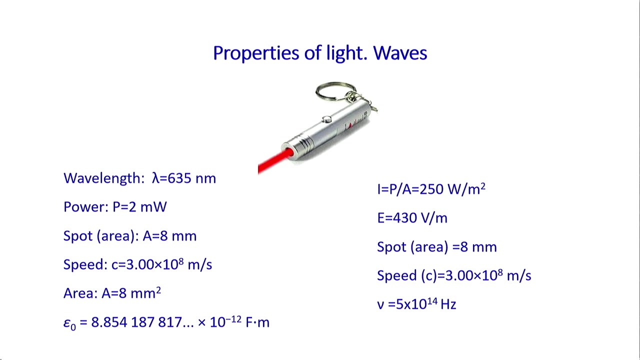 Irradiance is only when you take into account the area, Then maybe confusing, but it's an equation of definition: The electric field. using this and the equation I showed you before, you can calculate the electric field of the laser That is very, very, very, very high intensity. 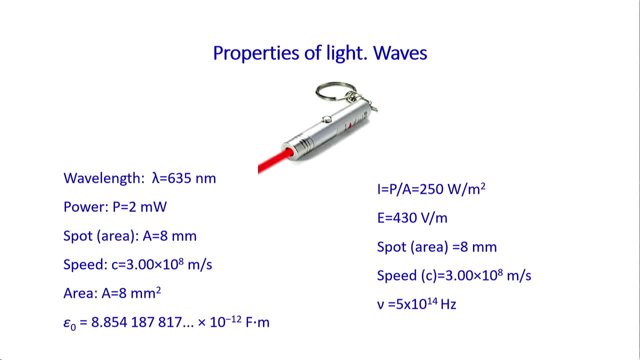 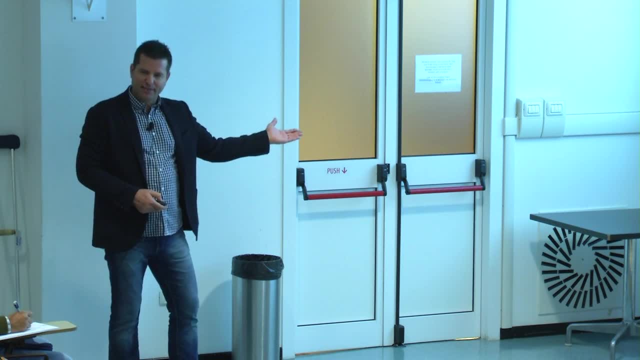 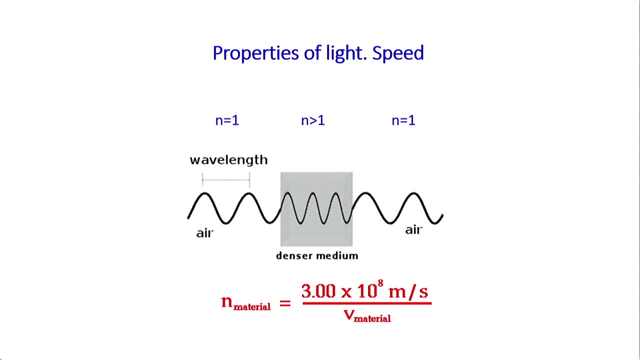 The spot area, The laser, The laser, The spot area, for example, and the speed of light that mainly we will use in the last equation for calculating this. Okay, Also, let's we speak about the speed of light In vacuum, in air. we know that the speed of light has this quantity that I showed before. 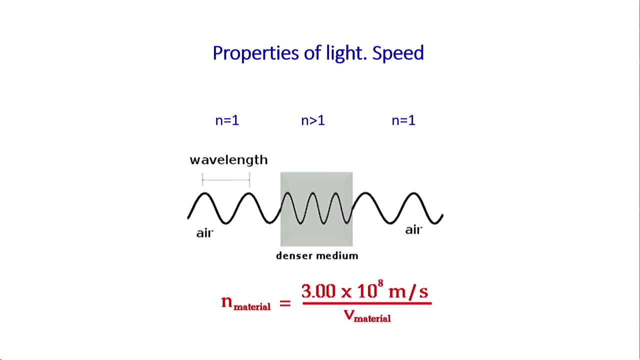 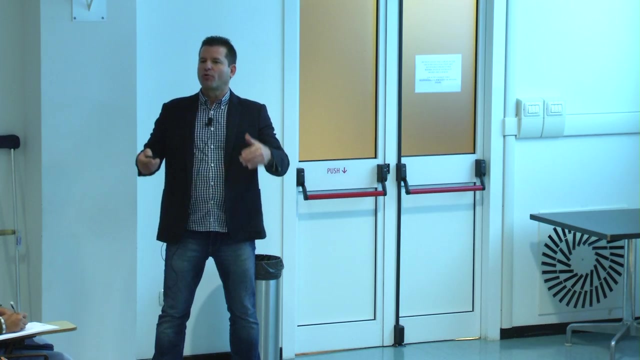 But when the light meets a medium, the speed is reduced. The light changes the wavelength, not the frequency. the wavelength and the relation between these two speed of light in the air and the medium is what we call refractive index, And this is very important parameter that we will use in microscopy also. 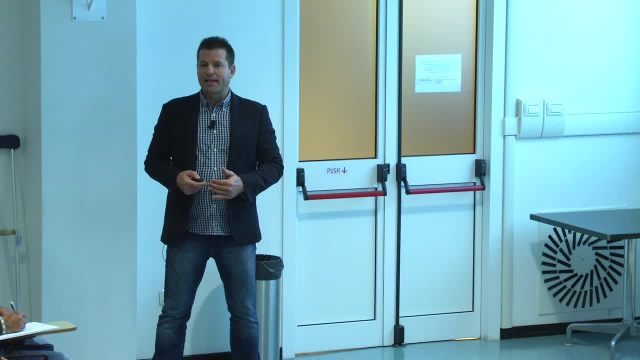 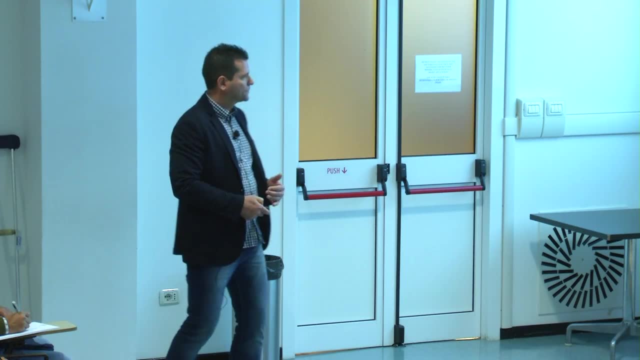 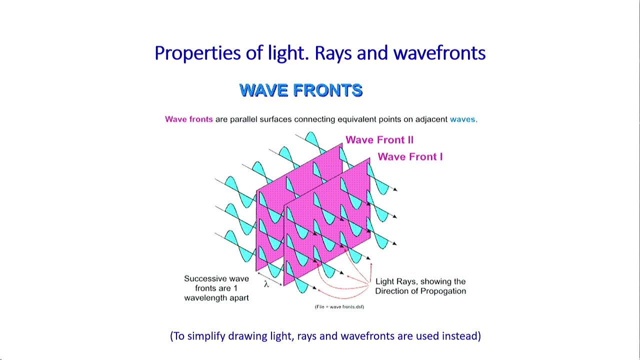 It's very important how we will select the materials for lengths and so on. Okay, Okay, And that's the process, using these equation, of course, But also it's very important in microscopy to start off with the definition of ray optics for defining the lens-maker equation, and so on. 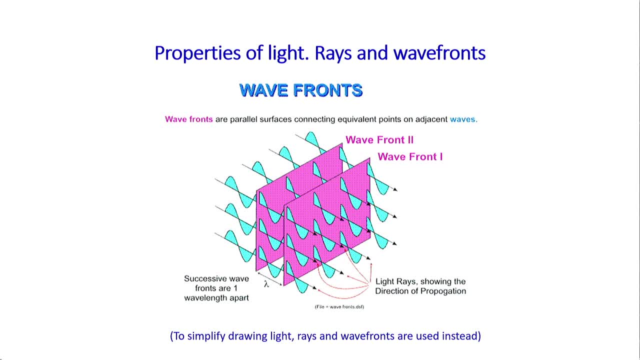 As I say you After that wave optics, But let's we look at the between ray and wave optics. Okay, wave optics, It's only a representation. We can when we have a wave, when we have a wave. 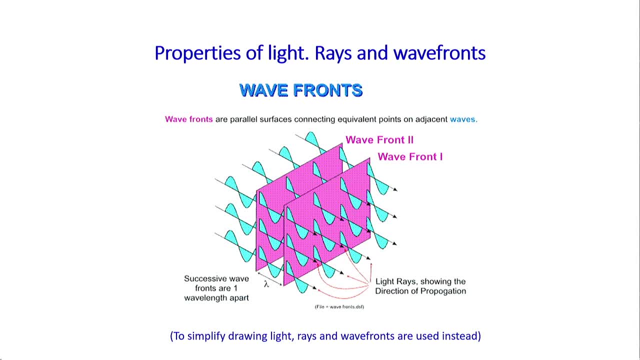 if we look at the points of the same, which has the same phase in the space and time, we call this the wave front. In this case we have a plane with wave fronts. This is, for example, for a collimate beam, we have a plane wave, But for a point source radiating. 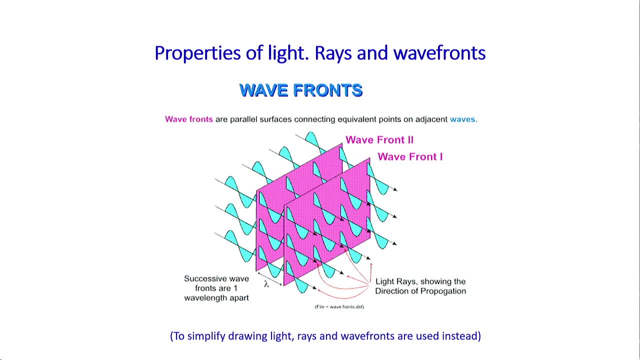 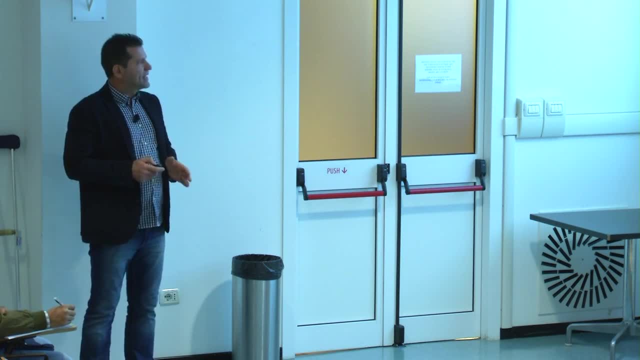 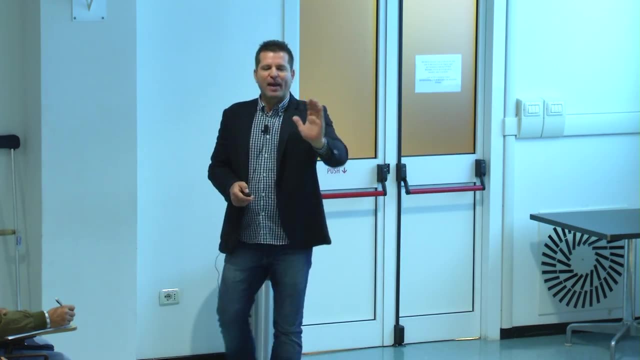 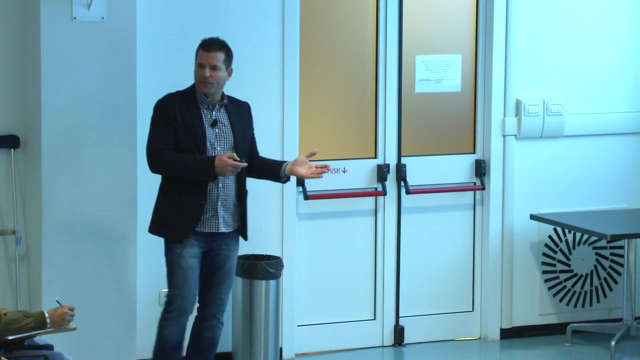 we have a spherical wave and we have spherical wave fronts as the phase of the same phase. If we represent this oscillation by this plane and the direction of propagation perpendicular to these planes, we will have a ray there and we can represent this wave also by a ray, by taking into account these concepts. 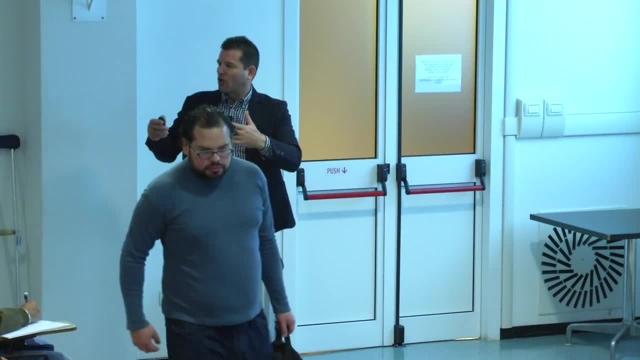 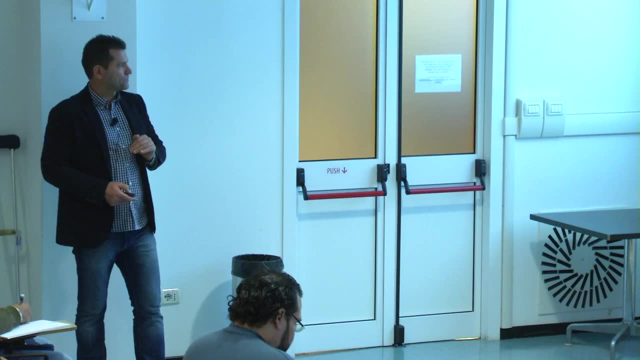 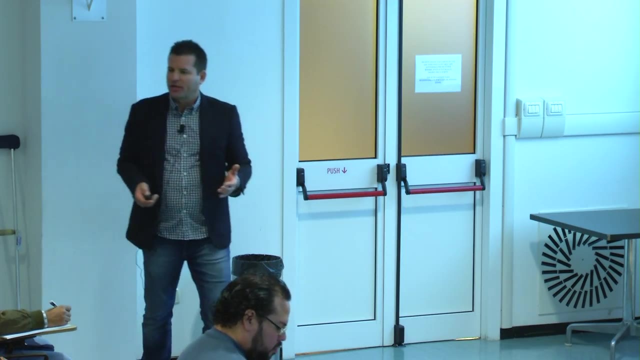 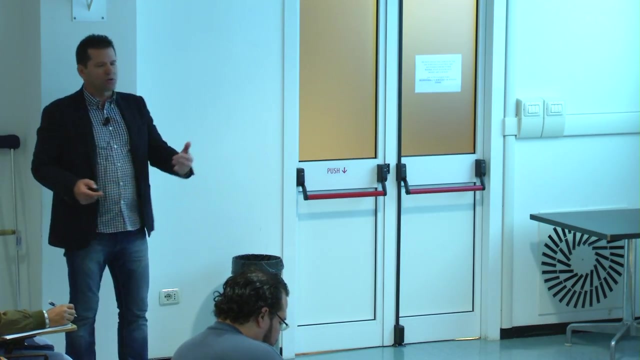 Also we know that the point in vector where the energy is going is in this direction, perpendicular to the wave fronts. Then this is only a simplification to better understand the theory of the ray optics and wave optics. But also it is very important to know light matter interaction. 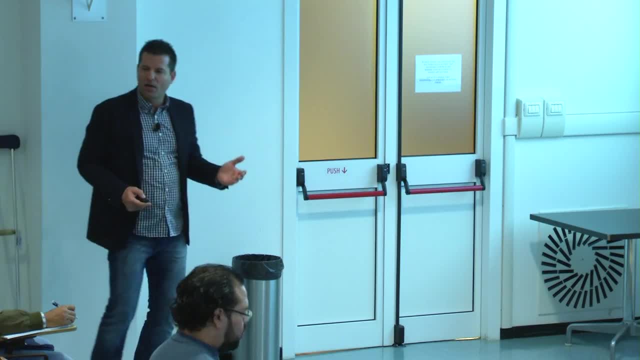 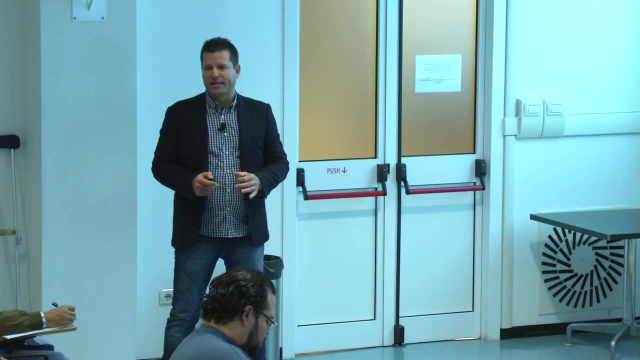 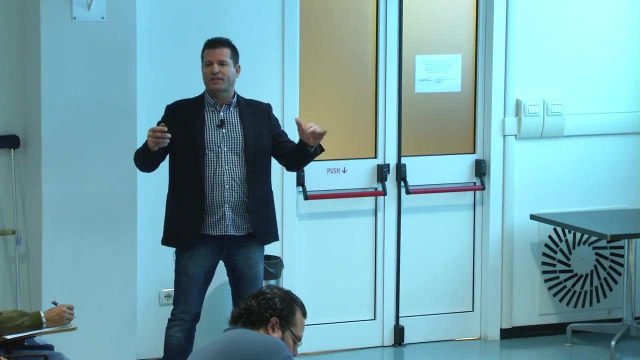 refraction and reflection, the Snell law, Because I mean what we can do to derive the lens maker equation and what happens from total internal reflection. all the processes in microscopy when we go to from one medium to another medium with different. 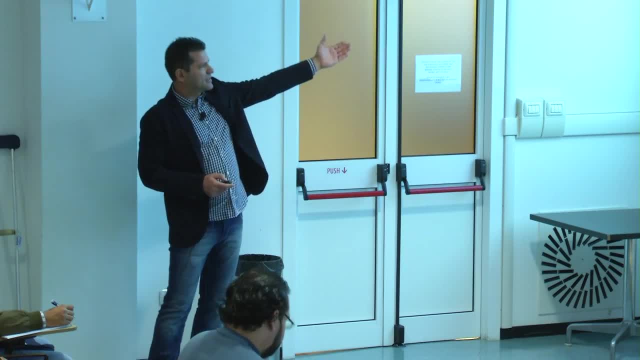 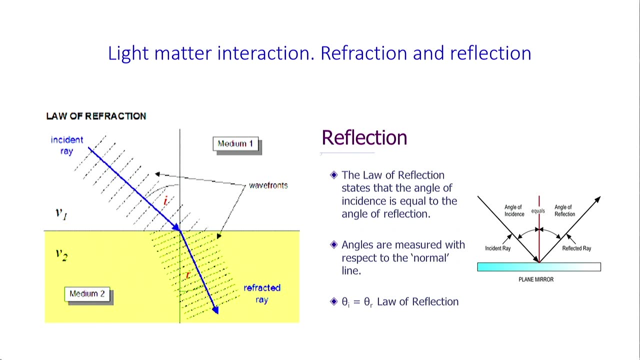 refractive results as many as we want to, we will be left with a range of, thanks to the dud practice index is to use the Snell law. What does the Snell law say? The Snell law first. the first point is that the law of reflection states that the angle of incidence is equal. 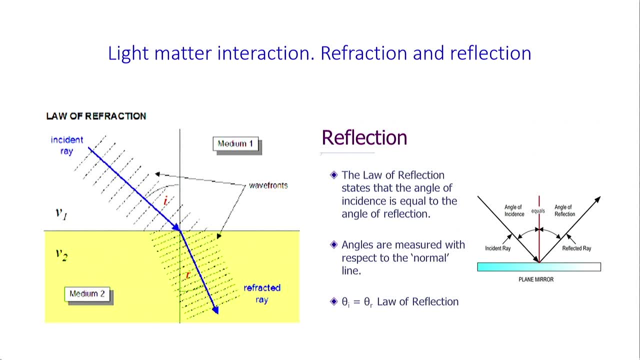 to the angle of reflection, as we can see here, And the angles are measured with respect to this perpendicular plane. This is the angle of incidence and this is the angle of refraction, and here will be the angle of reflection. This is the first stage of the Snell law. 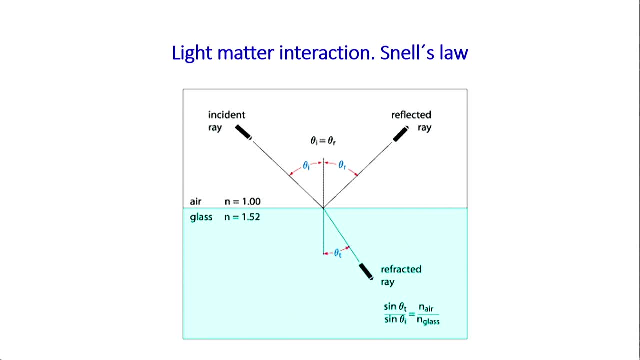 But the second step of the Snell law is that this, the relation, the relation between the angle and this angle, is through the refractive index of different media, The sinus of the transmitted angle times. the refractive index of the glass is equal to the sinus of the 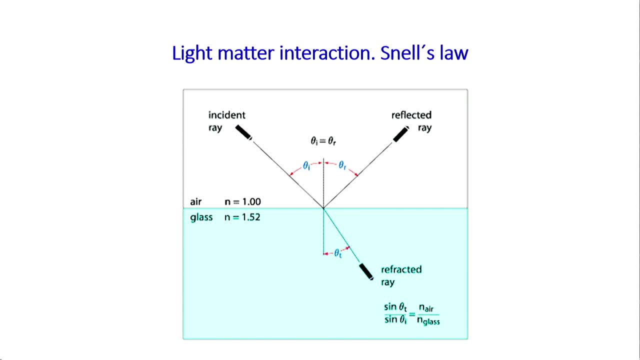 incident angles times, the refractive index of the air. if there is another medium, Then following the Snell law you can account for the direction of the propagation of the rays, But this Snell law only takes into account the direction. qualitative description For quantitative. 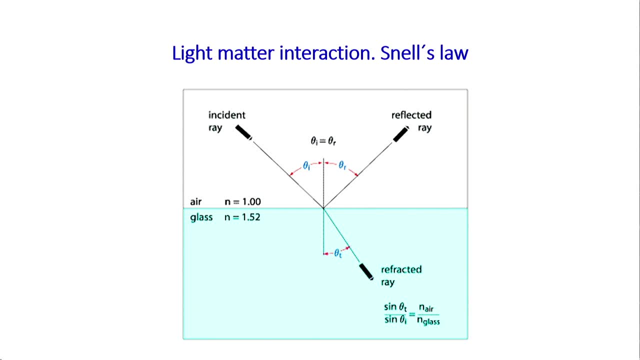 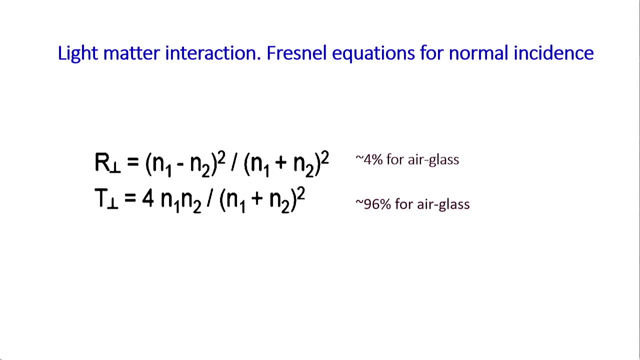 description of the amount of light going there, reflected or whatever you want, is the Fresnel equation, And there are different Fresnels, But I will concentrate only between the Fresnels equation for normal incidence, Because as we increase the angle, this is the reflection of light. 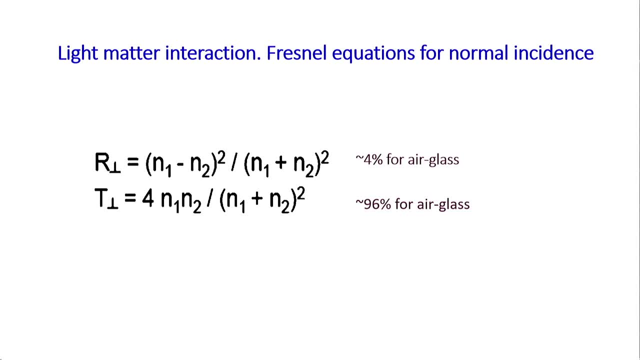 when we take into account normal incidence Under transmittance of the light, as we know, is lot of light. This is the angle of reflection timeập. So this is the angle of light. As you know, this is the angle of light period and this is the angle algorithm of light. This is a remarkable effect ofaged indicators. If you see the micro book slide here, you will see that there is a light break. the light is transmitting light through infrared light and yellow light. All right, And that's a metaphor for experience, And paired noir streaks fore long term record. Thedess a to some decide that the crypto society. 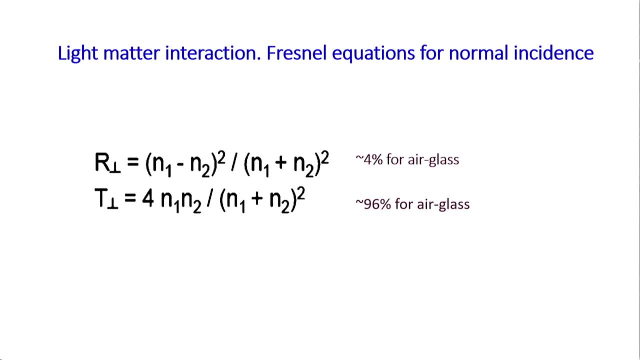 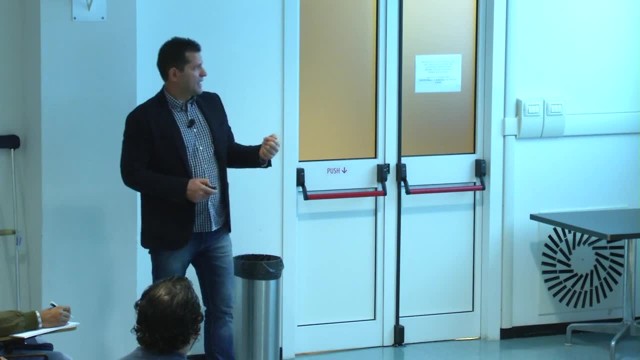 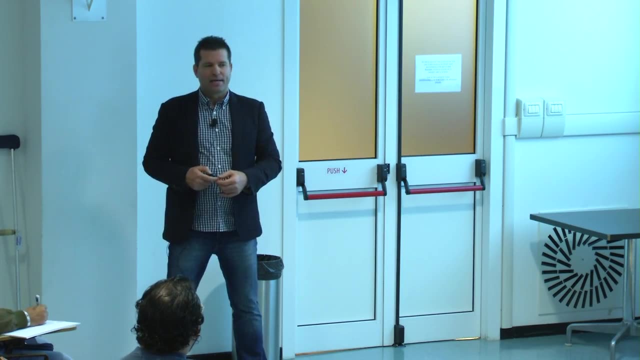 have normal incidence, 4% of the air glass will be reflected in each surface. But if we can change this proportion, we change the angle And there is a con for that in the Fresnel equation. You can look at this, but for now, with this, it's enough. 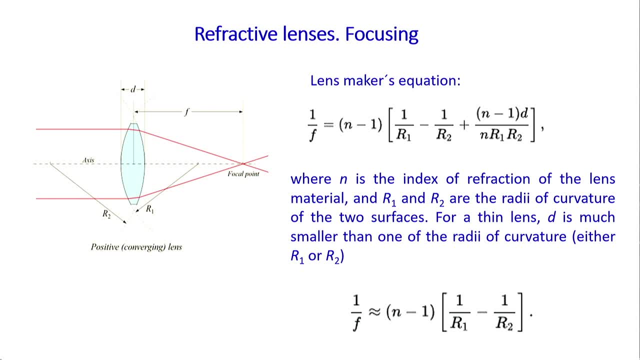 Also refractive lenses and focusing and lens maker equation is very, very important in microscopy. and this is the lens maker equation. Normally we build a lens using two surfaces and with these two surfaces that has different angles. And also here a con for the refractive index medium of the medium used here for the lens. 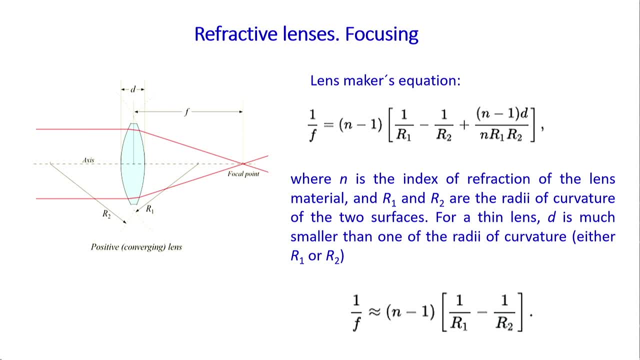 and the distance here between the top of this surface, But normally we use a definition called as a thin lens, In which this is zero or almost zero. It works very, very, very well for some definition in microscopy and in optics, And then we obtain this equation, which is a very, very good relation. 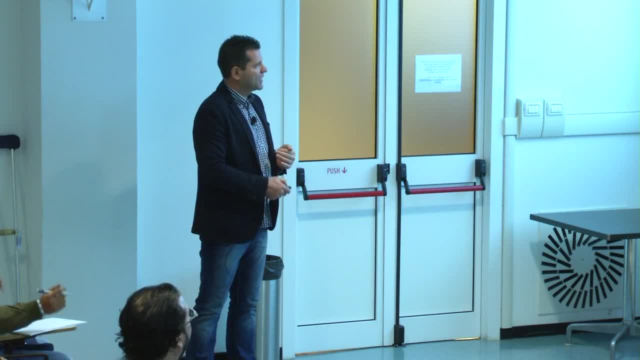 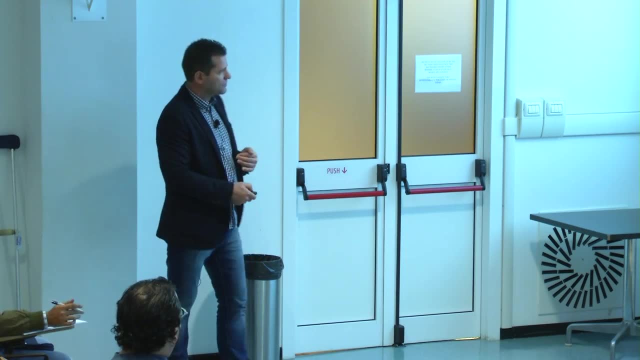 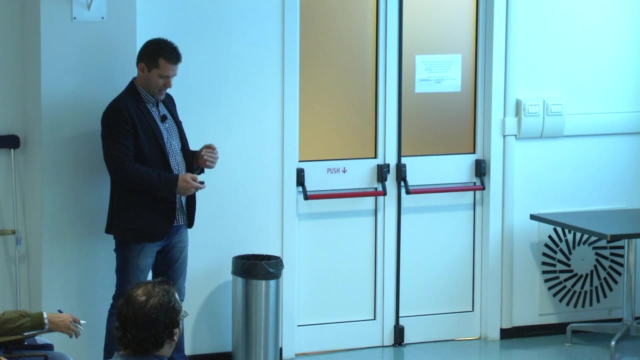 a very good approximation between the focal lengths of the lens, the refractive index of the medium And the radial index. The radial index is the focal length of the lens And the radial index is the focal length of the lens of curvature of these lengths. But we can have different kinds of lengths depending. 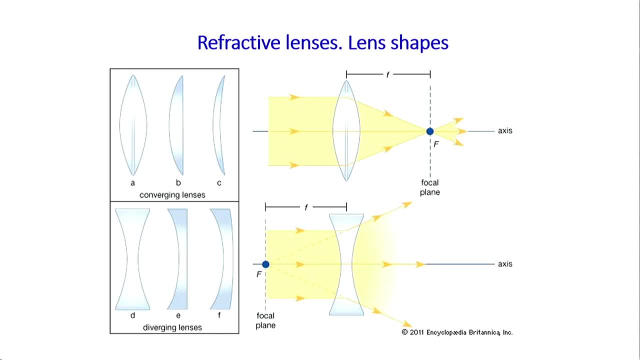 on the surface we are using there. For example, we can have converging lengths, positive lengths in which we can focus the light, But we can also have divergent lengths if we use two concave surfaces or meniscus with a plane and concave surface of this kind of meniscus. 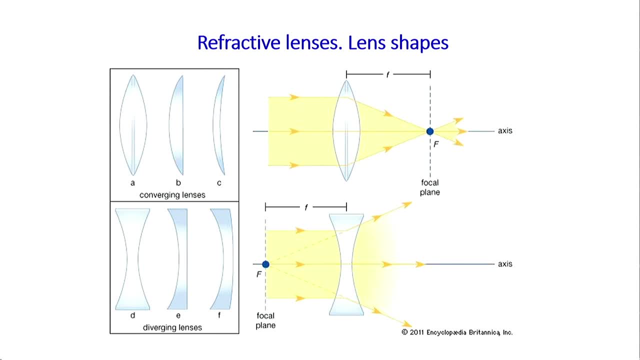 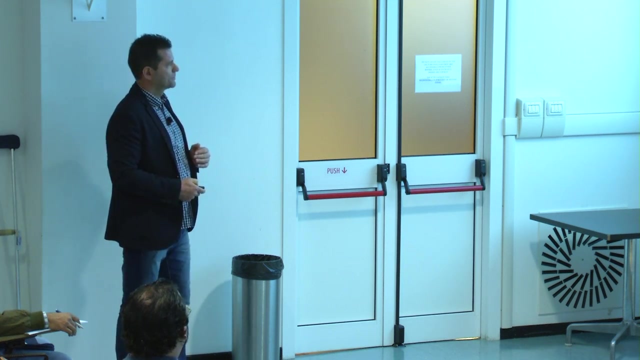 and every kind of length. Keep this in mind, because when you build an objective, what you use is this: a combination of lengths. So for chromatic and spherical aberrations, you use a combination of lengths, and this is very, very important, Only to keep in mind. 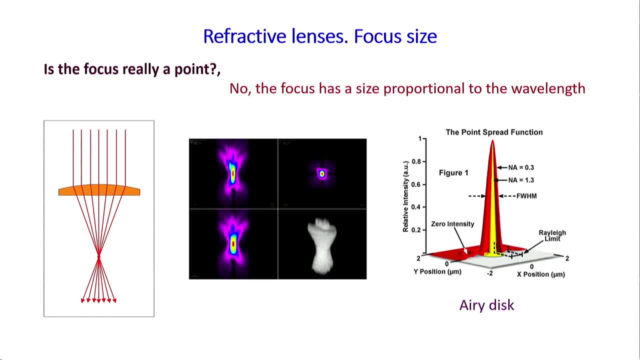 But also I say to you that wave optics is very important. Let us ask: is the focus really A point? when we focus a light, is it really a point? The equation is no. Why not? Okay, because the light has a wavelength. 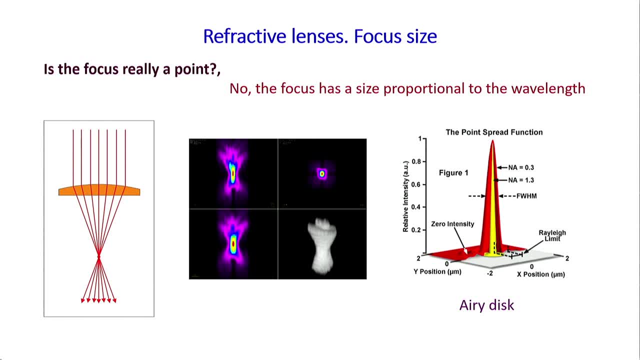 It's not a ray And we have diffraction. of course, that is related with the limit of diffraction in microscopy And this is what we will have in the focal point of the lens. This is the point spread function. We have there some distribution of intensity. 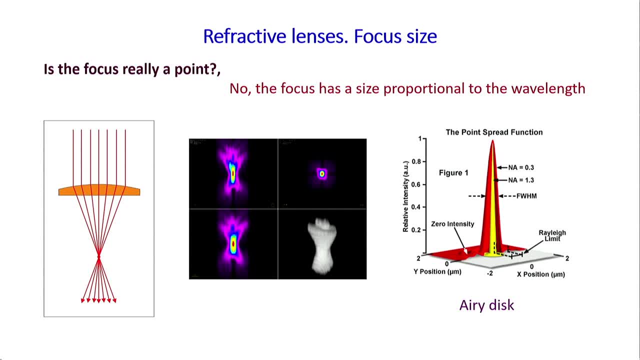 I think Miguel also will be speaking about this Distribution of the intensity there. That normally is. I read this, Okay, I read this: some minimum and maximum. This is the. I read this, And this is called the point spread function, And 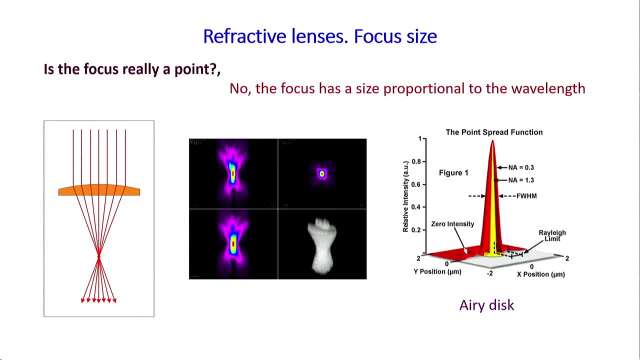 Of course we will see in the lab also the importance of this And in each lecture we will be remembering this, because this is related with the resolution. Of course you have a point there. You can resolve any component in the cell. 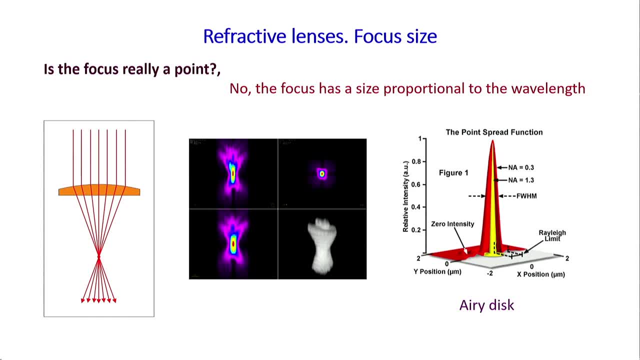 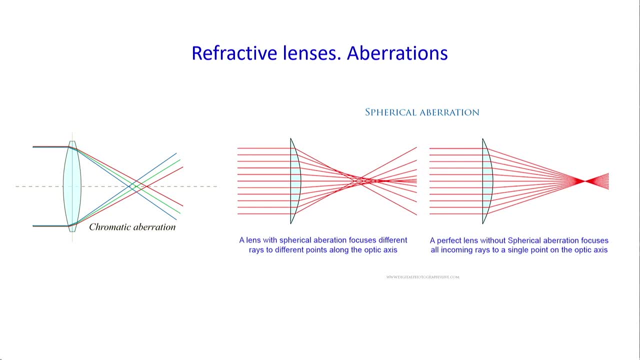 But it's not possible. You have a limit due to the diffraction of light. Then there are also- I will only mention about this- Miguel will derive this equation very precise: In microscopy, the main aberrations are chromatic aberrations that are related with the fact that different colors have different speed in a medium. 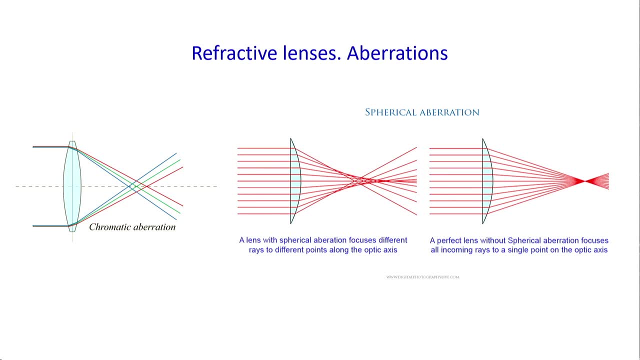 And different refractive index. Okay, Then they will be focused in different places. The red light will be focused there And the blue light before, And there we have a distribution of colors. How to correct that? Okay, Using meniscus, we will see that. 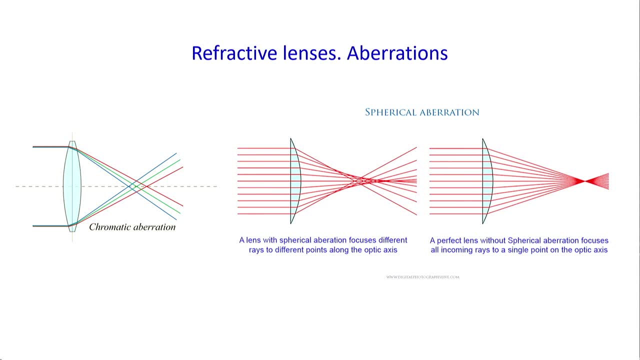 But also we have a spherical aberration That, as I say you, any surface is not the perfect focusing element And then, in any case, we will have aberrations. How we can correct this? Okay, For example, even using monochromatic light, we have a spherical aberration. 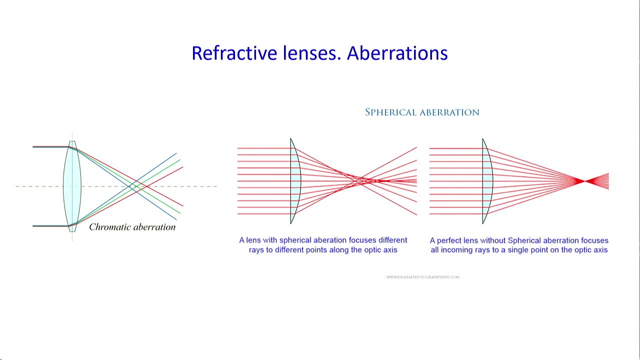 This light will be focused in different places. This is what I say about single lens. when we started, they started using microscopy. It was impossible to have a good image because we have different focusing The rise. The rise coming far away from the center will be focused far away. 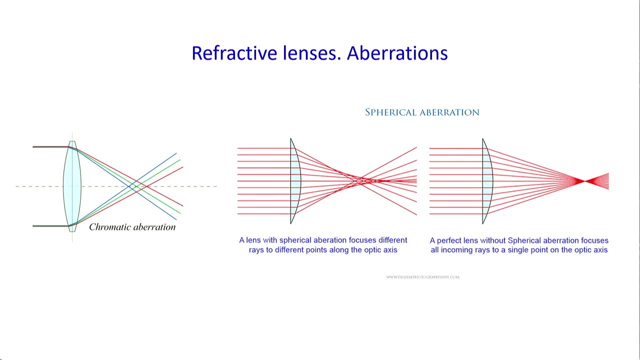 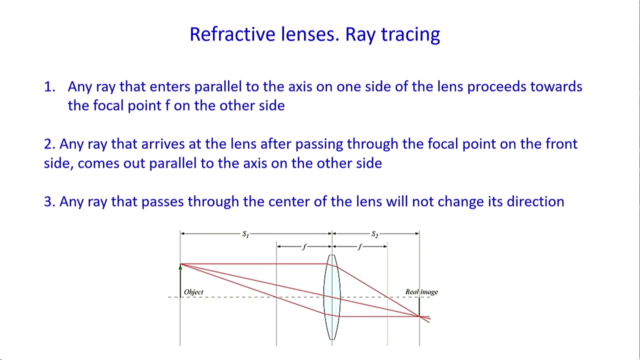 And the light coming here, they will be in different place. There are some techniques for correcting this, For example, correction colors. I will show you right now about this. But let's we continue with ray optics And let's we explain about three important laws for image formation. 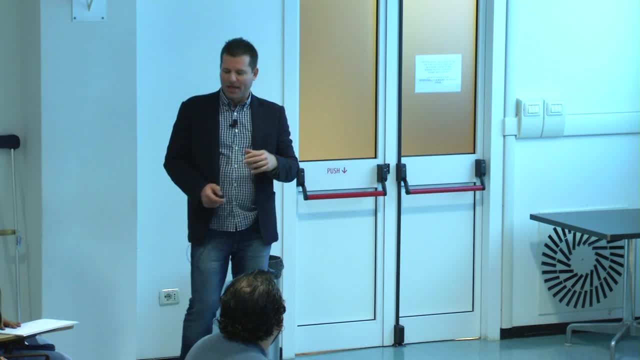 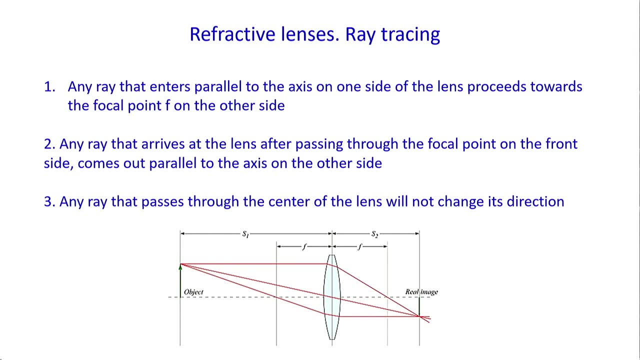 I will repeat it many times because it's very important. The first law states that any ray that enters parallel to the axis, to the optical axis of the lens for one side, proceeds towards the focal point of the other side. This is the focal point. 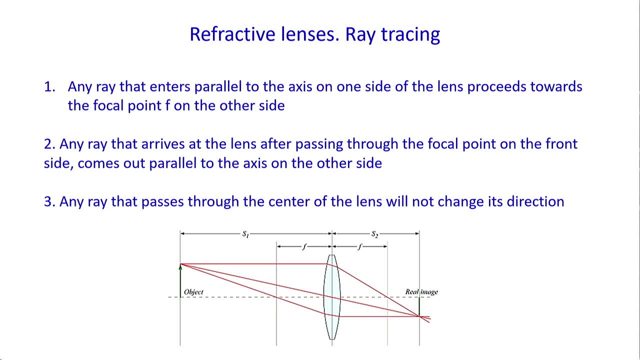 Towards the focal point. The second law states that any ray that arrives at the lens after passing through the focal point, through the focal point- this is the ray through the focal point- F focal distance will be comes out parallel to the axis on the other side. 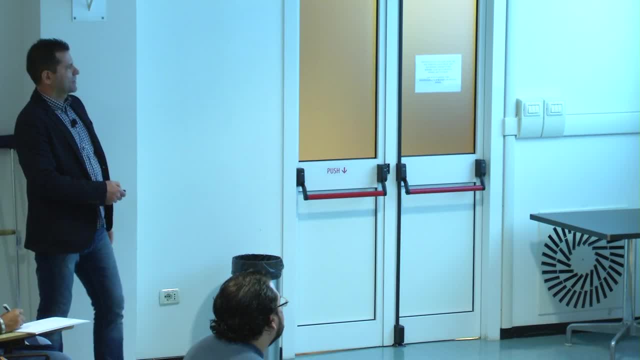 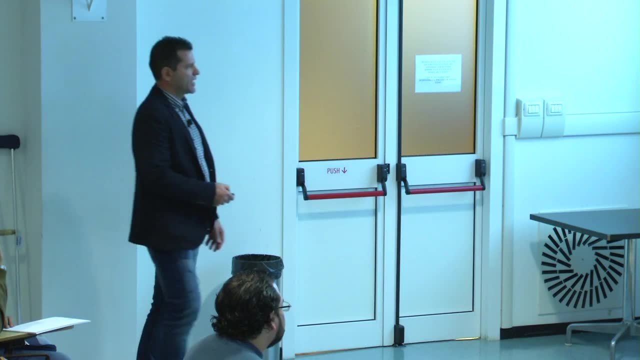 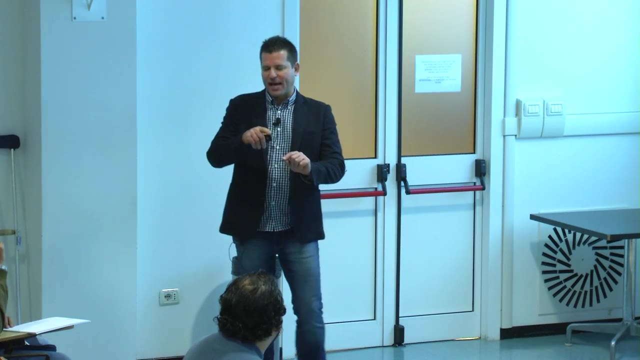 This is the ray And the third law: Any ray that passes through the center of the lens will not change its direction. Oh, if you have thin lens, of course change, But as this ray changes, but again, they are parallel. 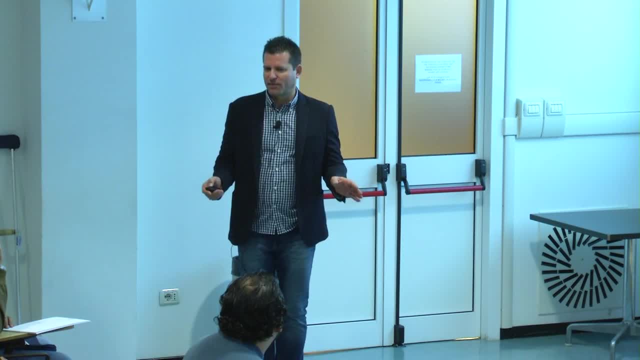 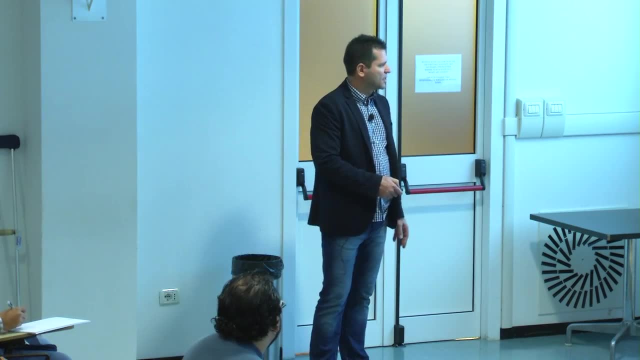 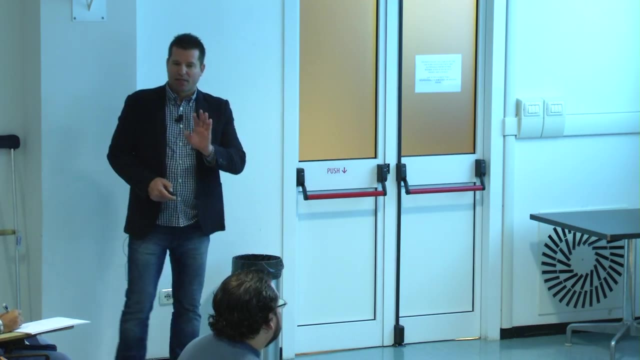 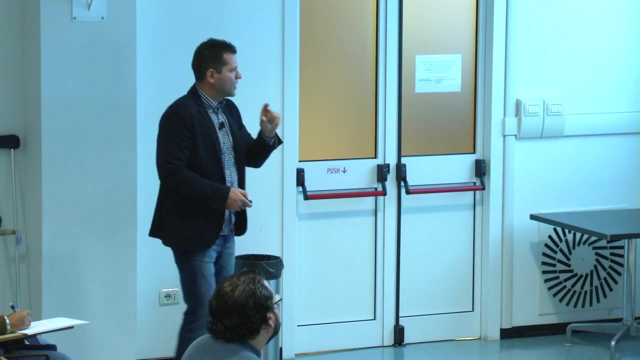 And you can consider it's a good approximation that they are not changing direction. And then you can build the image- The image here depending on where you add the object- Using these three laws Very, very simple: Not only the image, also the size of the image and the magnification of the image. 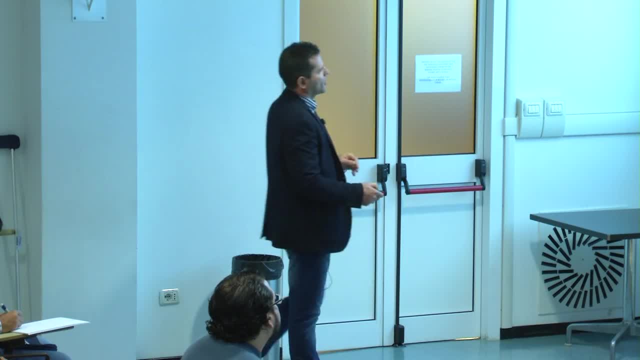 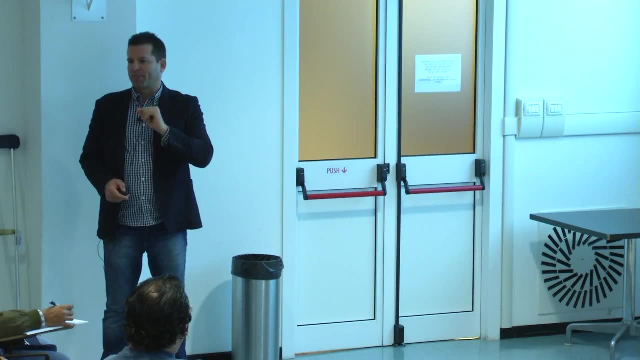 And this that is also called thin lens equation is very important. And you will test in the lab With a rule. You test there. This is the object distance. This is where you put the object far away from the lens. You measure there this distance. 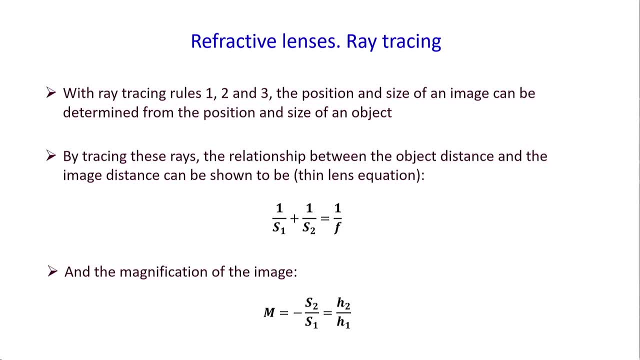 And this is the distance where the image will be created. This is what you need to know. And the focal length of the lens. You know that. If not, you can look there. And well, you measure with the rule And you substitute here. 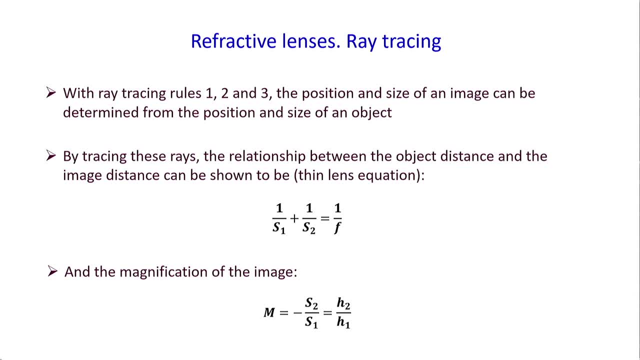 And you get where the image will be created, Which is very important Because there you will put your CCTV camera, for example, For imaging. We will do that in the lab. But also the magnification is related with this distance. The magnification is related is the ratio between these two distances. 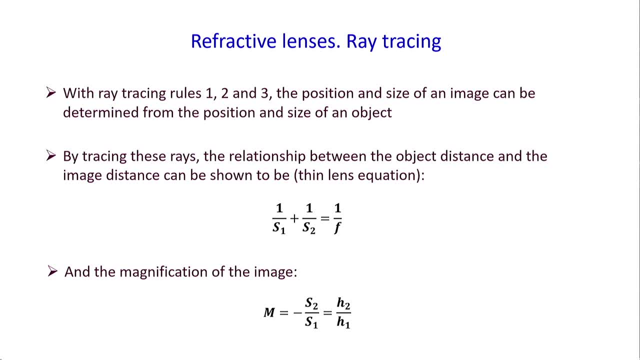 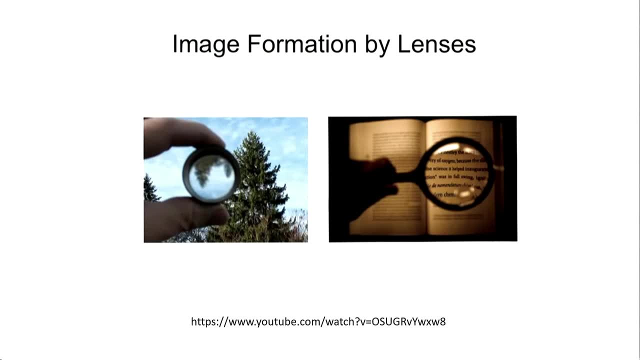 And also the height of the object. The object is related with magnification. But let's, let's we think about. This is what you were asking me. When you look with a single lens very close to the eyes, What you see is this: 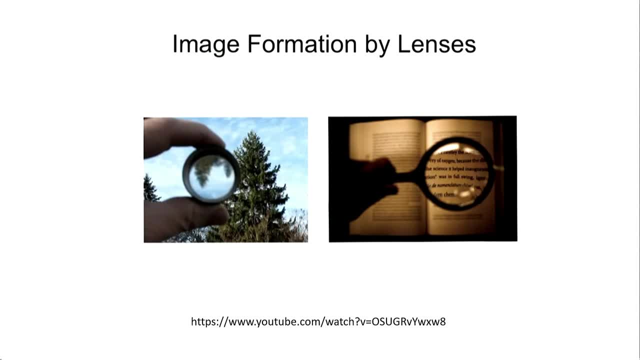 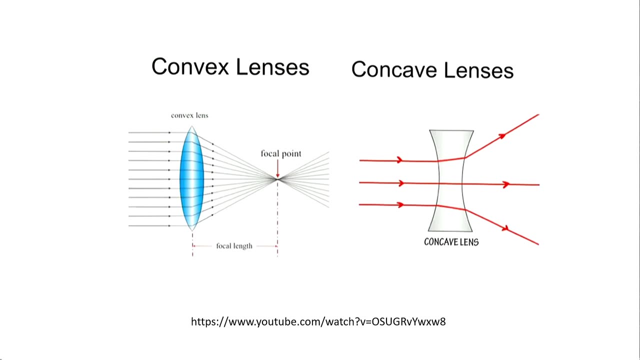 You see there a right the image. This image is between the lens and the focal length. You look at virtual image. Due to that, you can see the right image. But in this, in the other case, You look at the real image as inverted image. 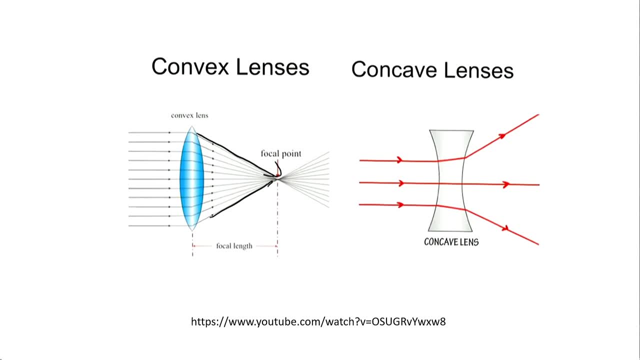 In the other case because the image was far away. But let we look at image formation. This is the first law. Parallel beam of light will focus the light in the focal length. This is for the first law, But for the divergent lens. 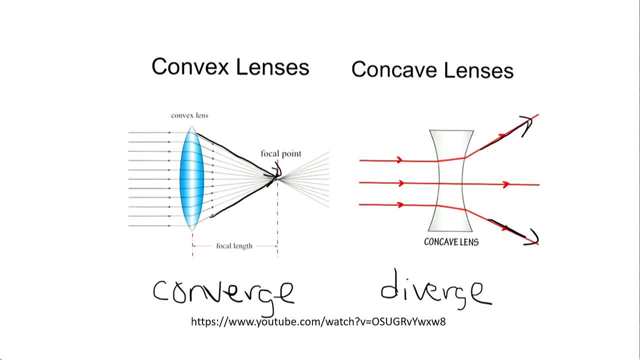 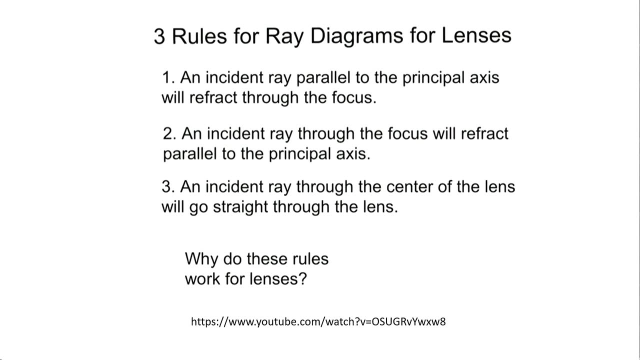 The parallel beam of light will diverges, And this is also very useful, As I say you. I will repeat this many times Again. First, Two And third: law Of image formation. Okay, Let's we follow this. There are many, many videos in internet. 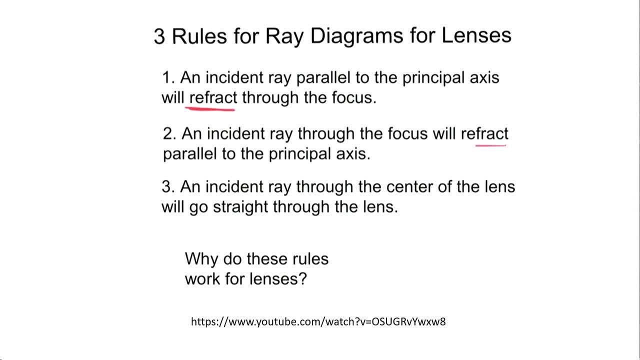 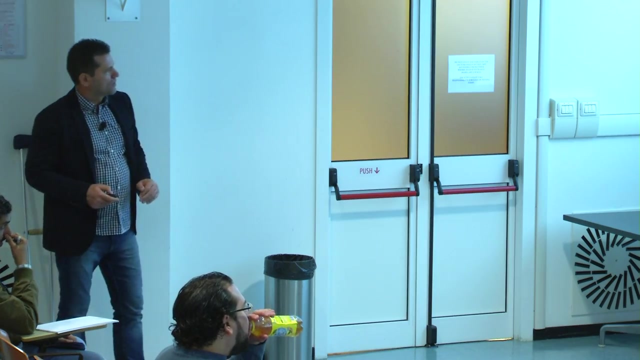 Showing this. I encourage you to look at this And check this every day. And then Google practice in the lab. All this law, But after we are in complete knowledge of this, We also of course, as I say you, The Snell law for the derivation of this. 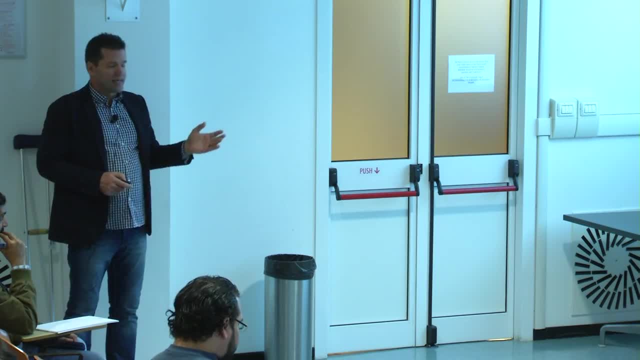 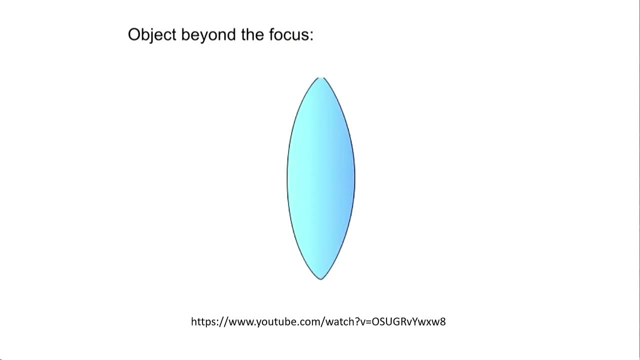 The Snell law that I showed you before Is very important, But what I will do now Is to add the object in different place, Even at the final of this video. I will show you another video And you will see. It's a kind of video that is in internet. 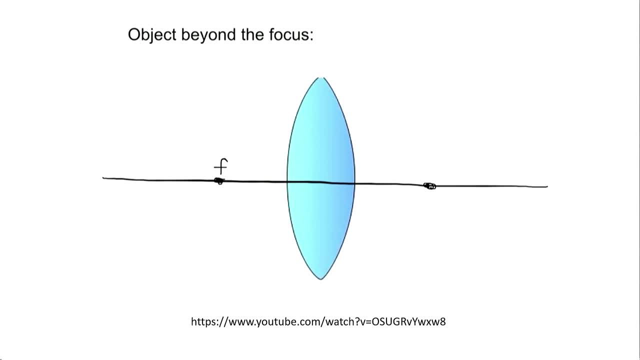 That you can play there Putting the image in different place, Because when you put the image In this different place, I show you the three rules. Okay, But now We will put the object Far away, For example, From this focal point. 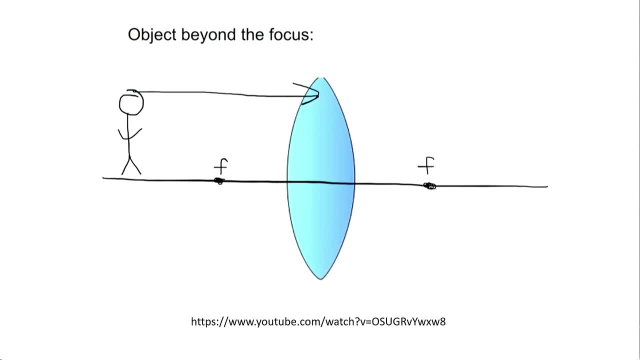 We put the object here. The first law Again, Right, parallel, Right to the focus. Okay, Now We apply the second law. The second law says We can use this focus, But as we used this focus before, We can use this focus. 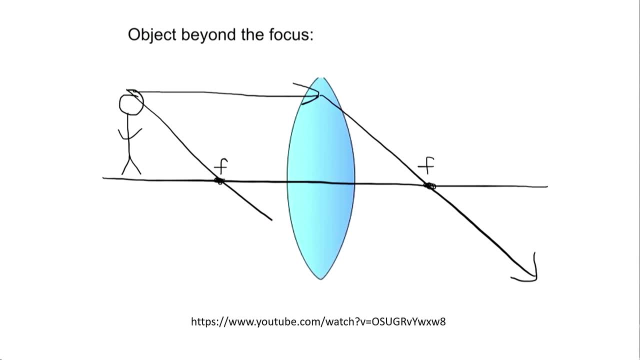 Like coming from the object Passing through, the focus Will be parallel. Okay, And we have now A point here. We have the tip of the image Here, But we can also use the third law That says Right coming up. 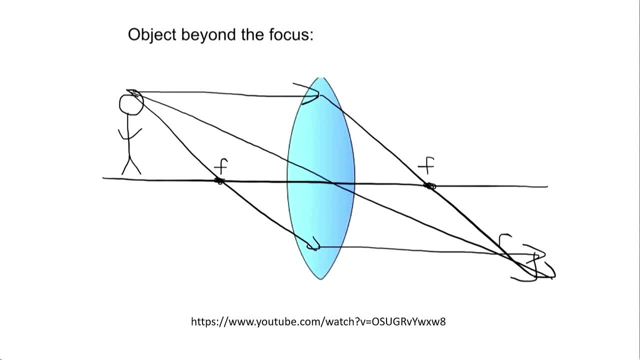 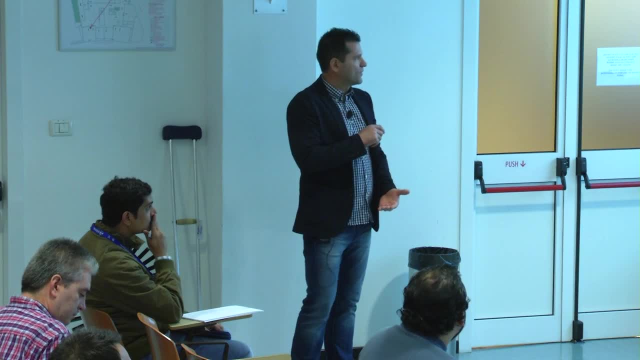 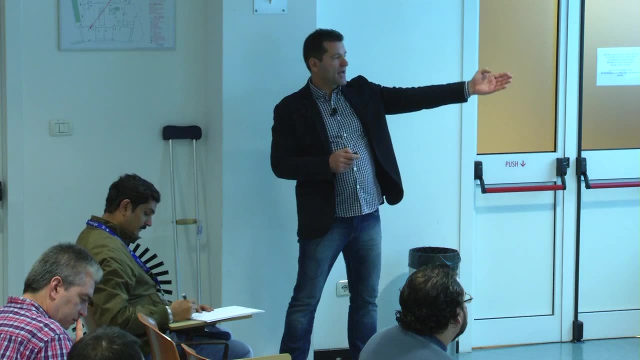 Will be without any change And then We can build The image There And we Also Account For the size Of this image. But We did Using The And is of course Real image, But inverted. 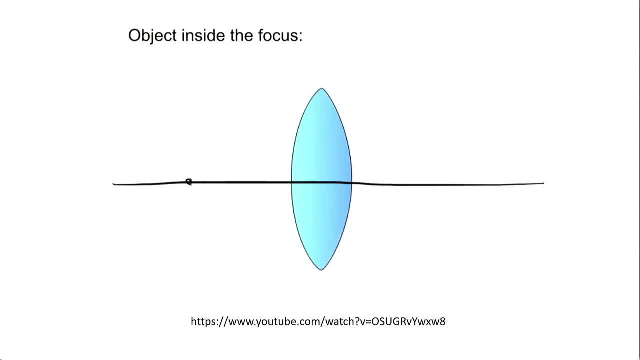 You can do also Using the lens maker equation, And you will account For this Size of the image And also for the, For the magnification of the image, Of course. Let's we add the image In between The focal length. 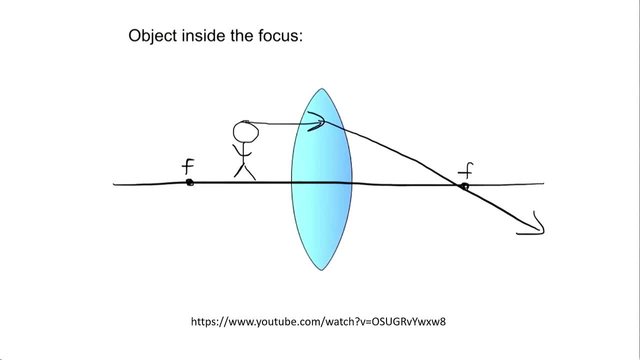 And the length. Now, Right, parallel, Right Through the focus. Okay, First law, Now The second law. Let's We use This Because We have used this before. Then, Right, Coming From the focus, 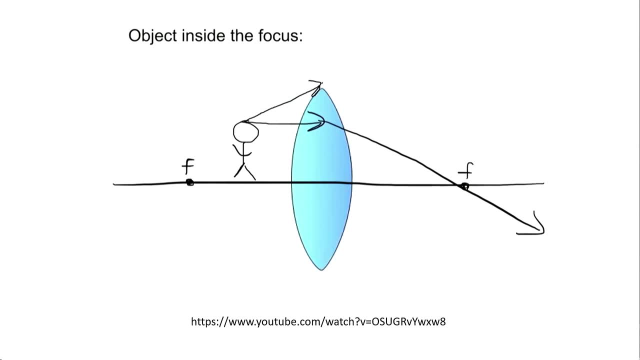 Right Coming from the focus Will be Parallel. Okay, Right Coming from the focus Will be parallel. They are Diverging. Okay, And the Third law, But We don't need The third. But 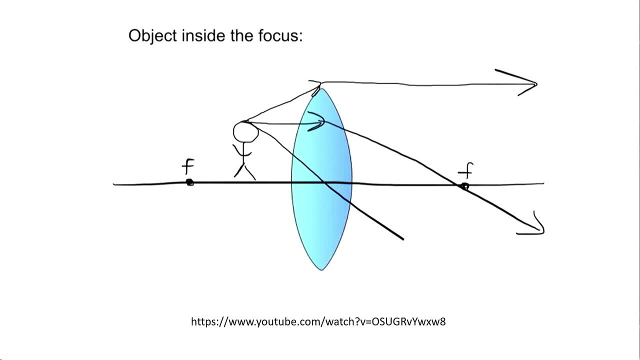 We can use, We can decide here. Okay, The third law Said: Okay, Also diverging. If we Continue This line Back And we Get All together, There We have Where the image Will be created. 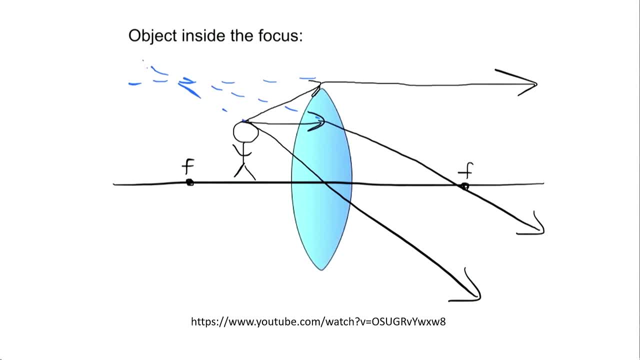 But This image You cannot see. You, You look At this image And you look At: There is An object, It's a Virtual image, It's not Real image And it's Also Amplified image. 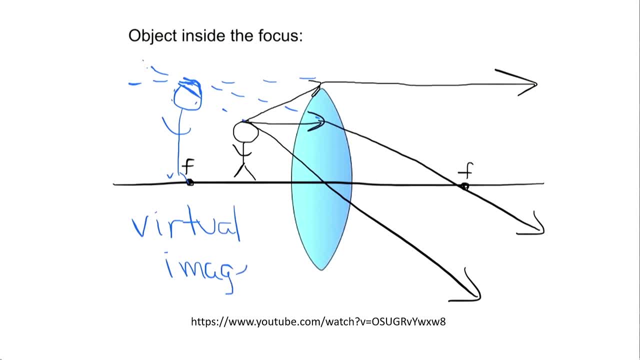 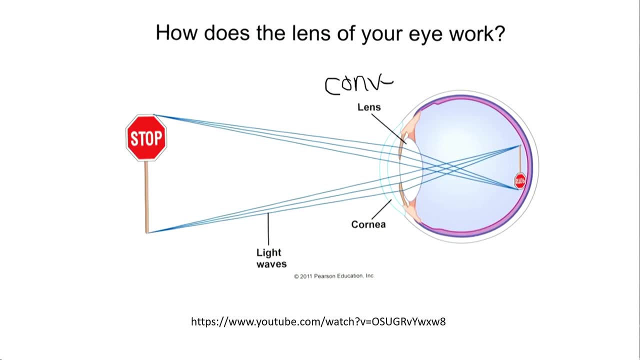 It's magnified Image. This is what Also We have In When we use Also Divergent Divergent Length. Okay, This is Also What Happened In Our Eyes. 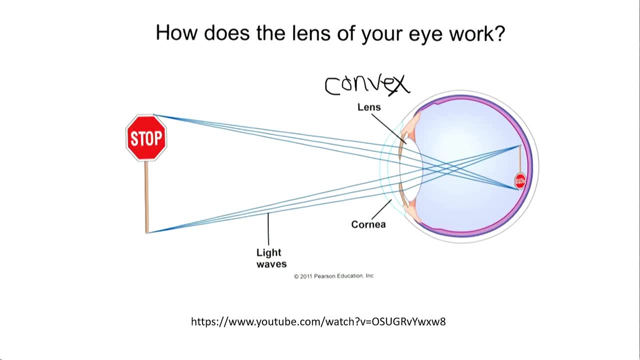 In Our Iris, When We have Different Beings Coming From The, From The Eyes, Then This is Very, Very Important Concept That We have To Keep In. 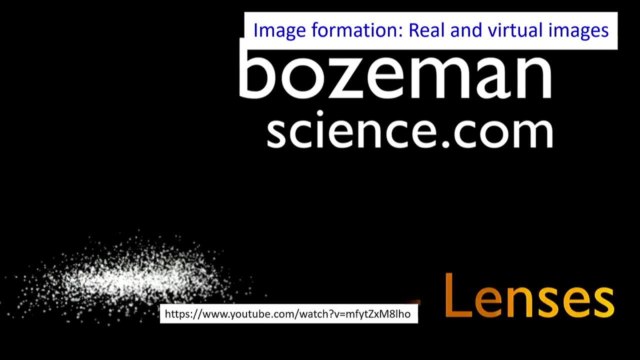 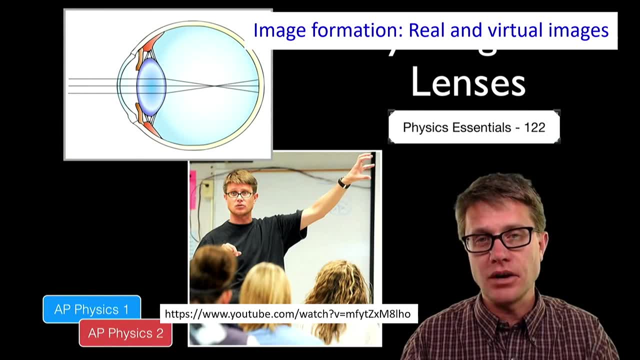 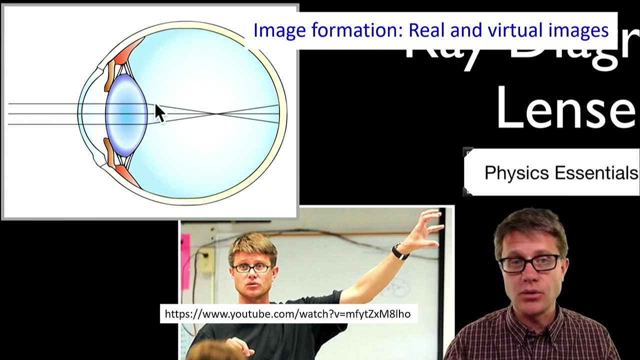 Mind And I Think That With That And This Video Will Be All, For Let's We Look At How We Can Create The Image In 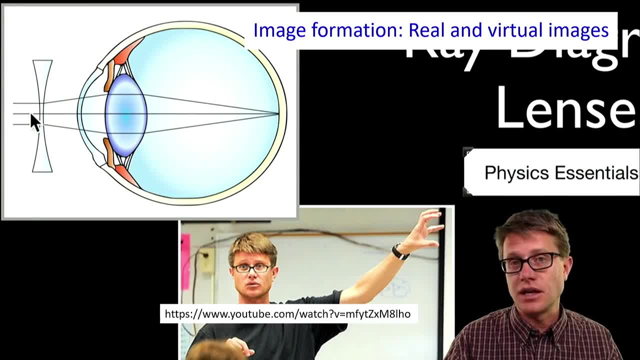 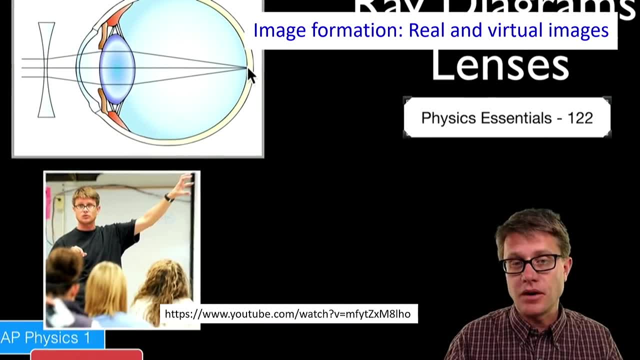 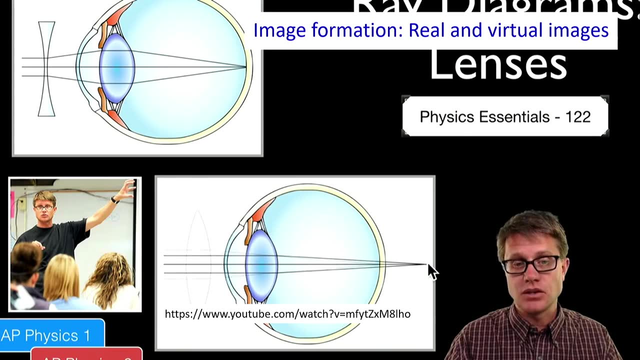 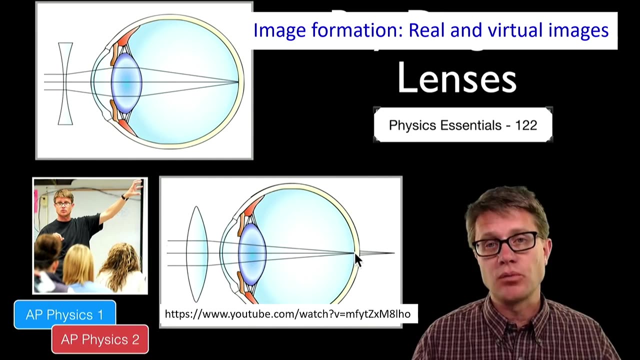 Different Place. There Are Some, Some Internet, Some Of This Kind Of This Video That I Encourage You To Use, This Every Day, Our Eyes. 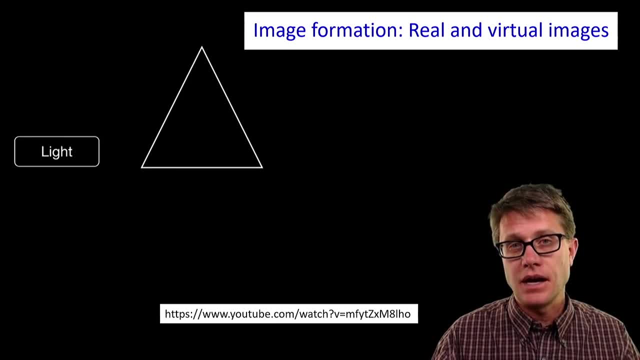 Okay, If The Light Is Focusing Before, Before The Retina, We Add A Divergent Length There And The Opposite When We Have Another. 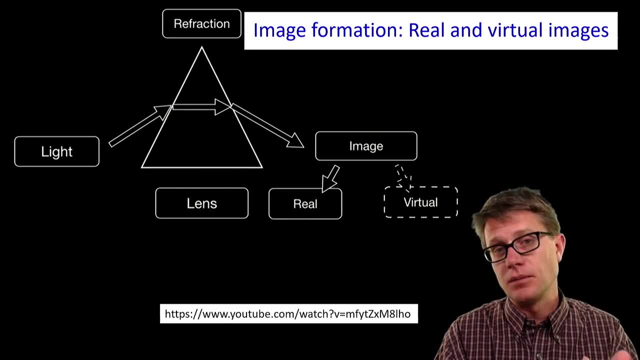 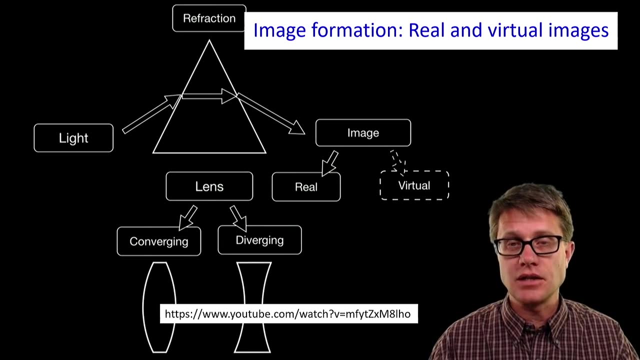 Kind Of Correction There What I Say Before, The Important Or The Basis Concept Of Refraction And Image Formation Using Length, And Now We Will. 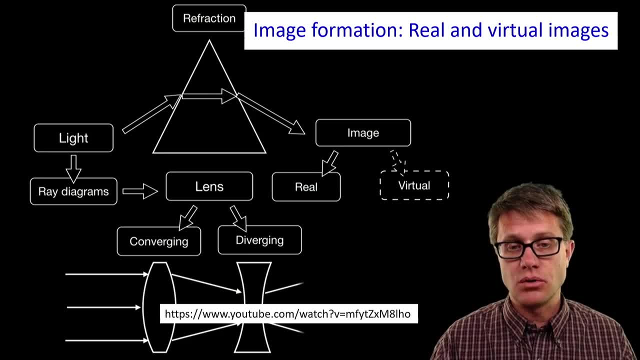 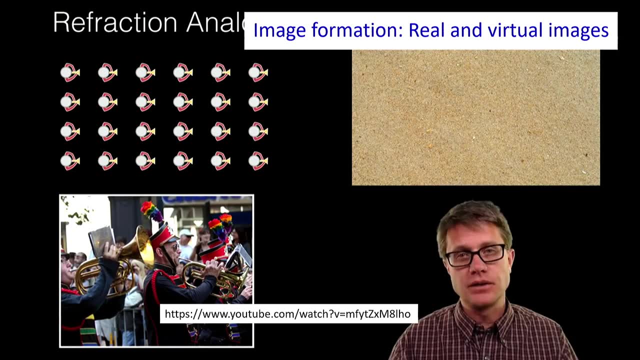 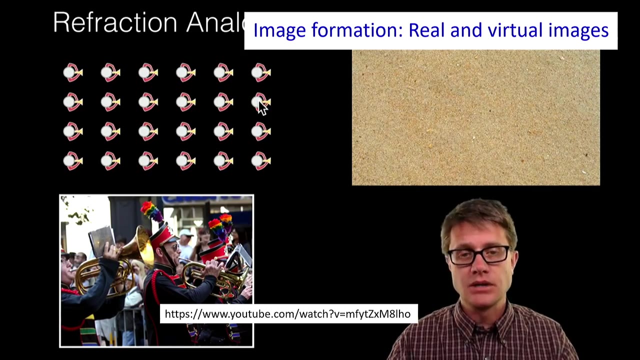 Start With Very, Very Nice, Very Nice Application On. He Is Explaining Here What Happening To The Light And Very Nice Comparison With A Group. 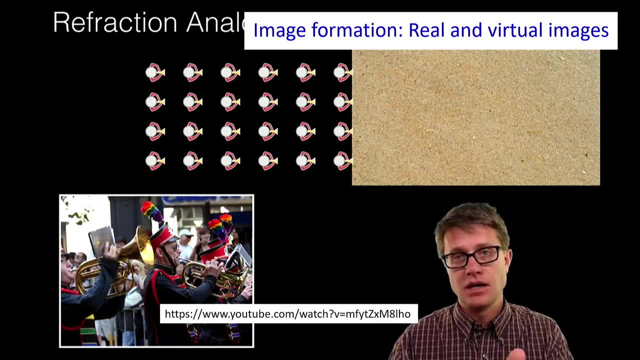 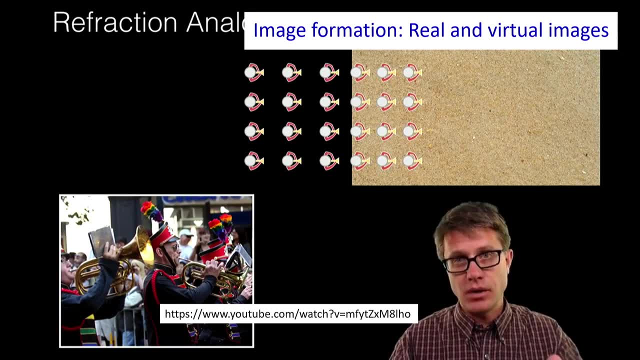 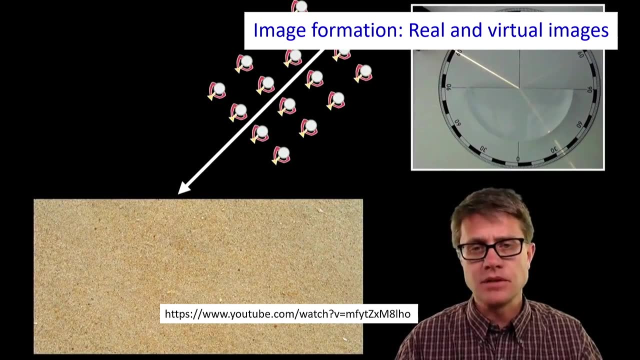 Of Musician- Military Musician- When They Meet An Obstacle, This Is What Happening To A Head- They Will Be The First Slowing Down. 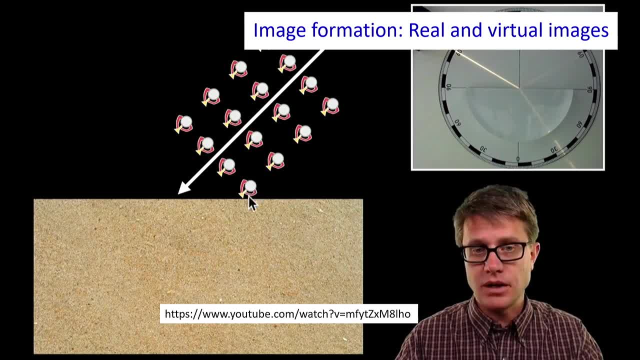 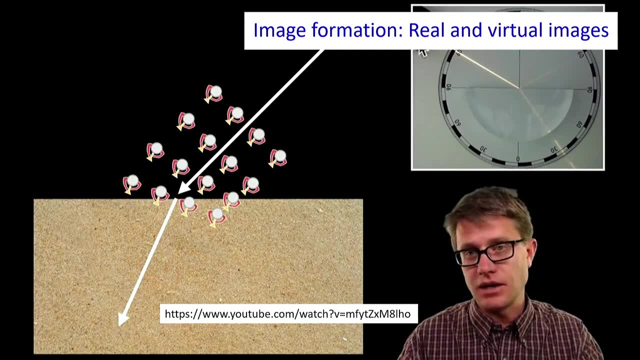 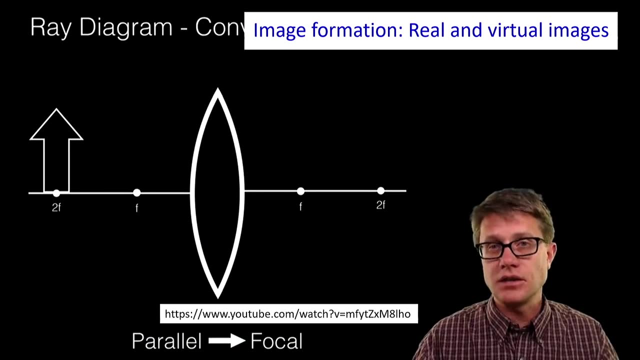 The Velocity, Then They Will Be Here Slowing Down The Velocity, But This Will Be Going More Faster Then What Happening In A Medium With 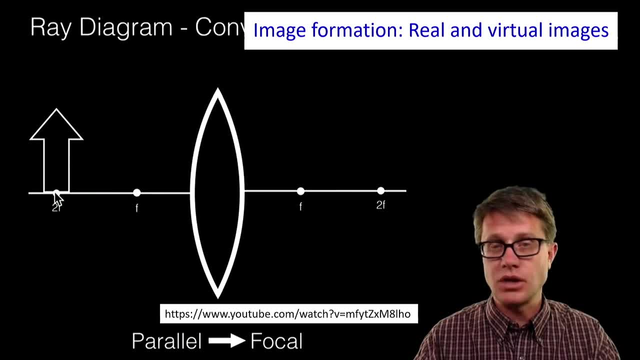 High Refractive Index. And Now Let's We Look At This Very Interesting Application About What I Said Before About The Three Laws. Look At: 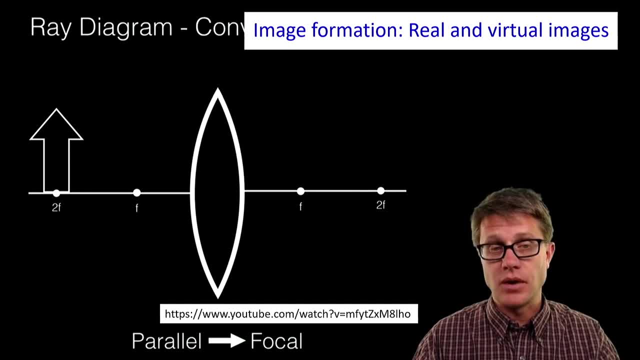 The Focal Length, Exactly Twice The Focal Length Of The Length With The Same Size. By The Way, We Have Very Nice Image Of The 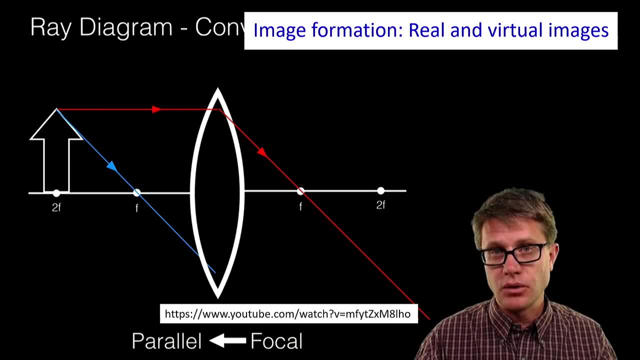 Face Of Albert Einstein. Okay, Light Through The Focus, Light Parallel, And We Have The Tip Of The Image And The Third Law, Only, Only Will. 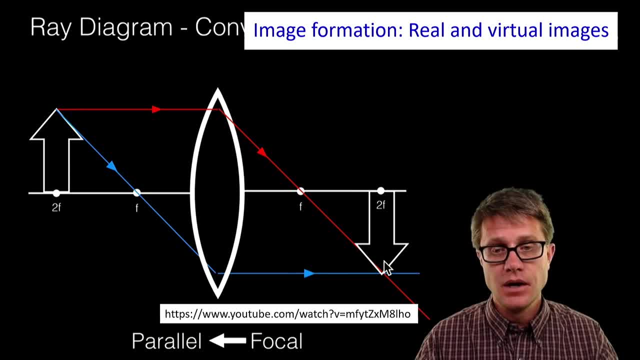 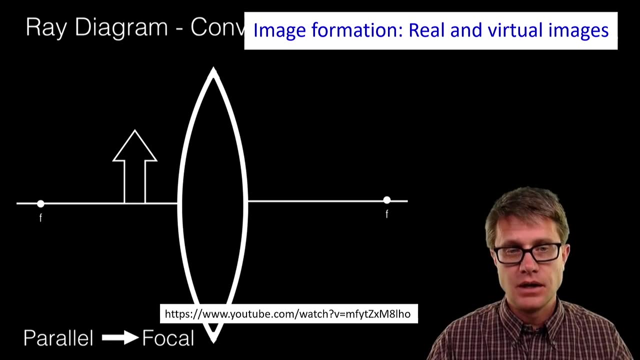 Confirm That This Is A Tip Of The Focal Of The Image, Of The Focus On The Length Of The ção, The Length Of The 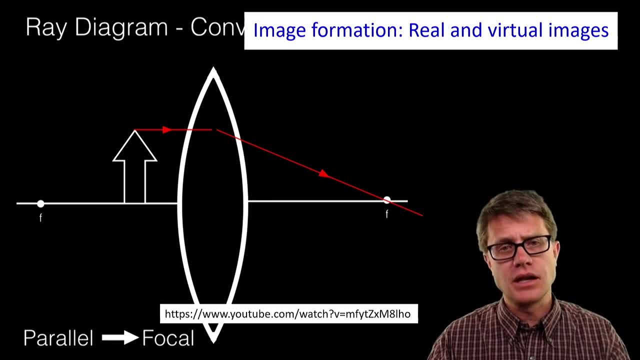 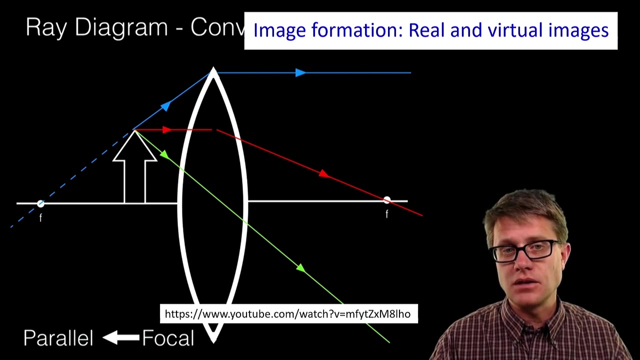 One In The Length Of Everything. Okay, You, So We Type From- goes parallel and we don't need the third ray, but the third ray doesn't coincide also, then we have again diverging the continuation back here and we have a virtual and also magnified. 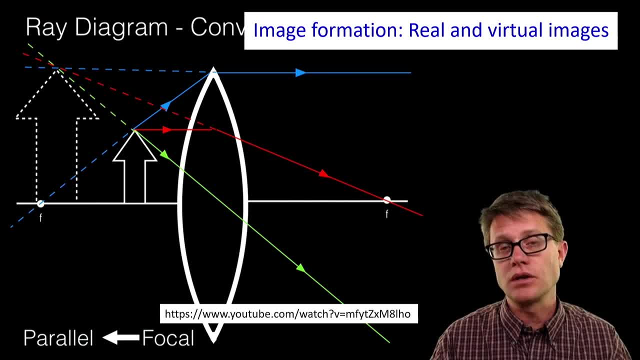 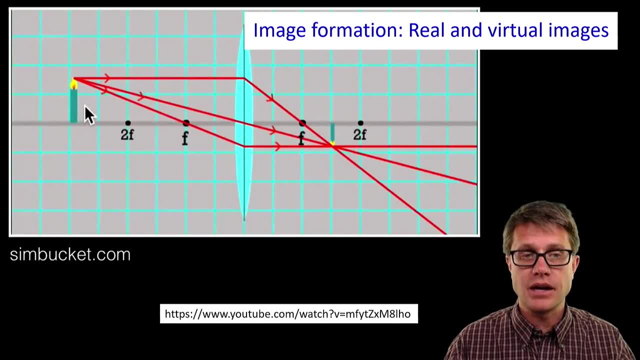 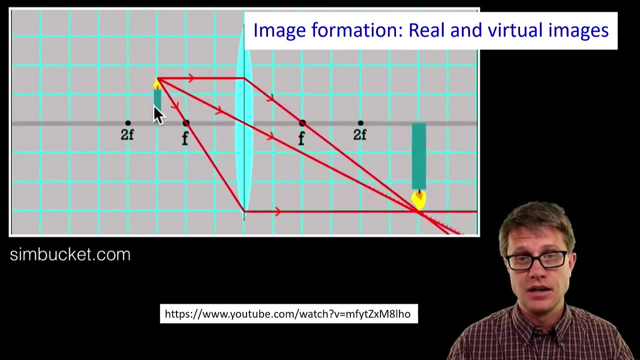 image of the object there. this is what we have. when we have a lens very close to the eyes, very close to the eyes, and we look at the book, we can see the image, not inverted. this is what I show in the book there: single lens, and this is very interesting. see what? 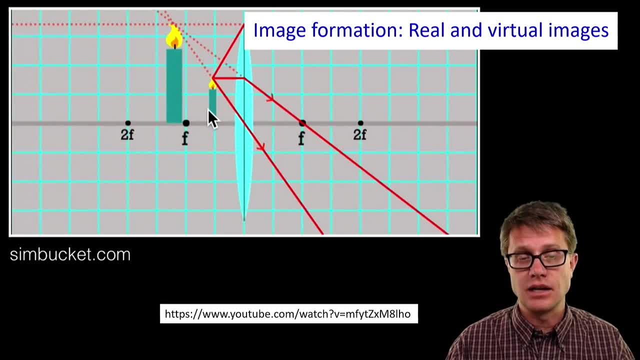 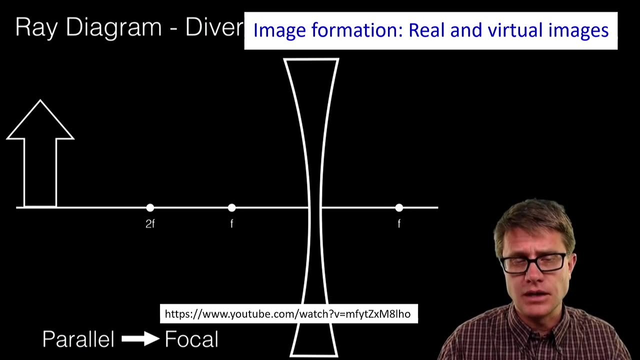 happened. when you move there, the image get virtual and then back, you create the image. this is a confirmation of what we said before And now, okay, he will show with divergent lens. divergent lens, again, parallel beam of light. normally we use converging lens, but also it's possible to use divergent lens. 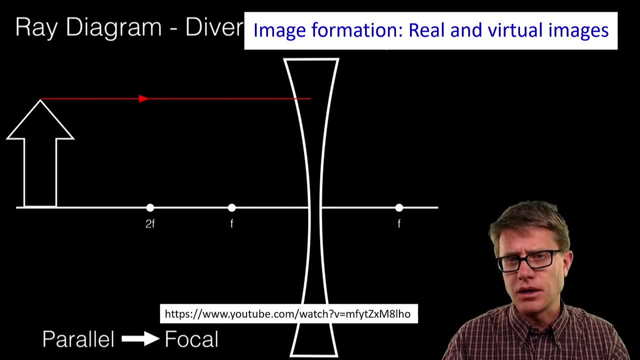 it's good to know about. Okay, Okay, This: when we use divergent lens, right, parallel, right, divergent through the focus, again the second ray, again through the center. no, any deviation here. we construct here from. 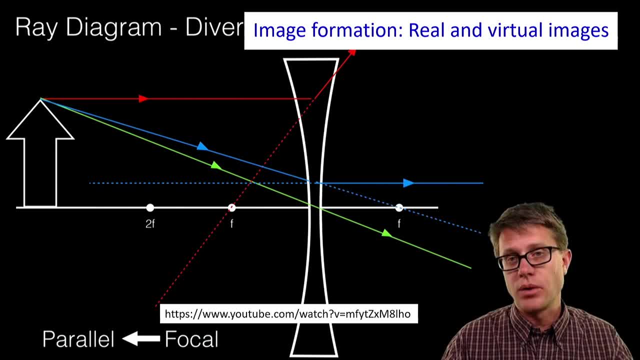 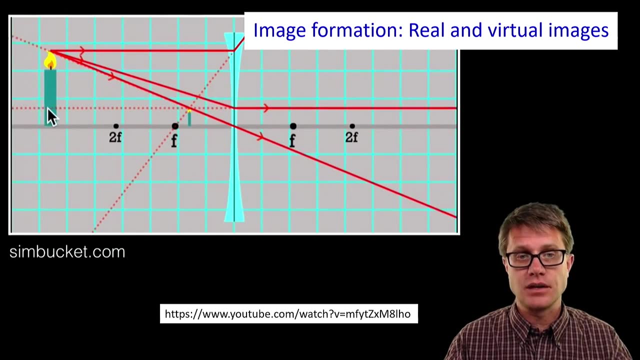 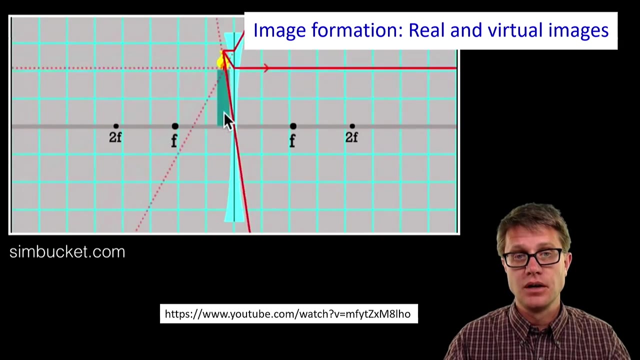 the focus parallel beam of light and we have this light and here no deviation. if the light is passing through the center, then we have an image. here We have reduced image and virtual. this is what happened. see what? how change the size. 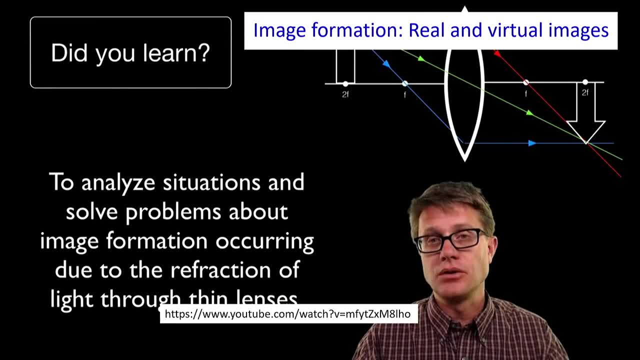 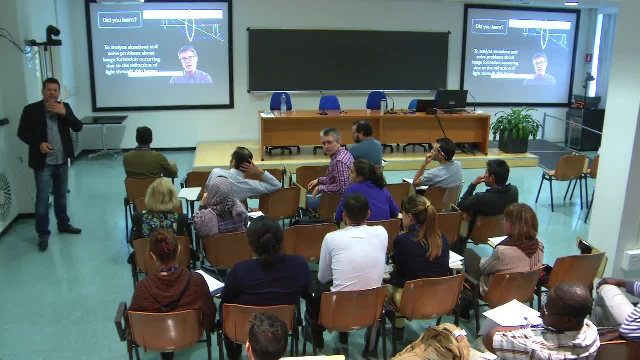 of the image when we move there. okay, Do you have time, Miguel, please send me? Yes, 12.38. Is 12.38.. Okay, We have still. We will know in a couple of minutes.